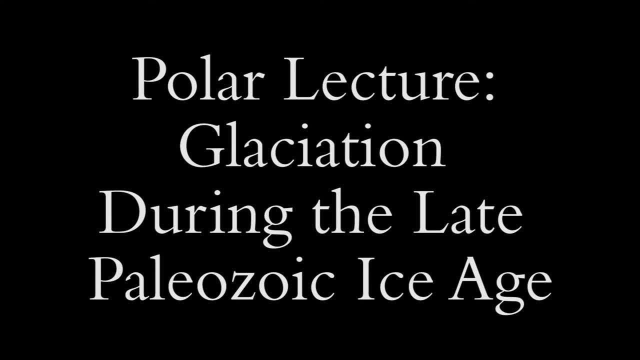 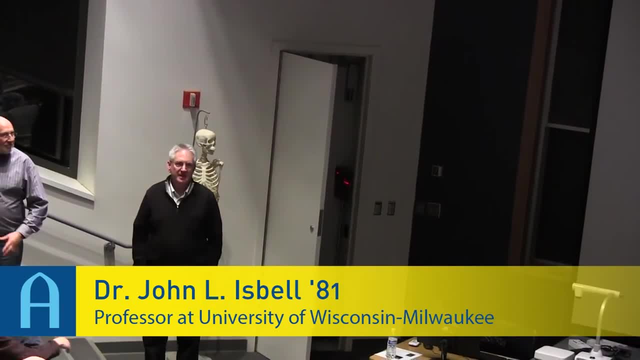 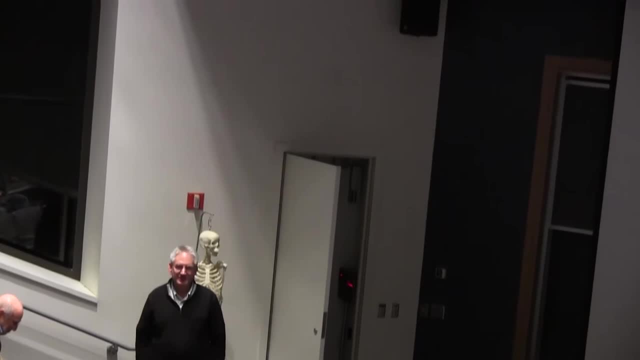 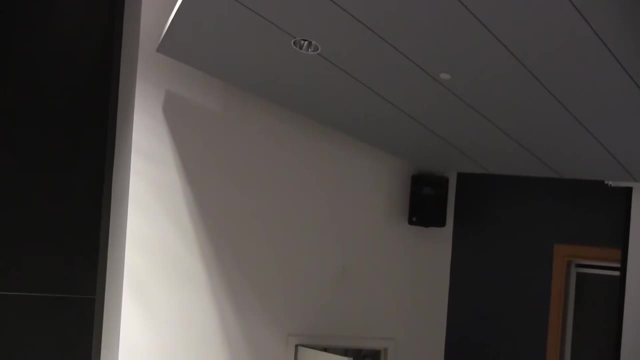 I appreciate Bill inviting me here. It's been a while since I've been in the department. I was here four years ago and I think it's been 15 years prior to that and it was probably another 15 years before that. So it's hard to believe that it's been 35 years since I graduated. 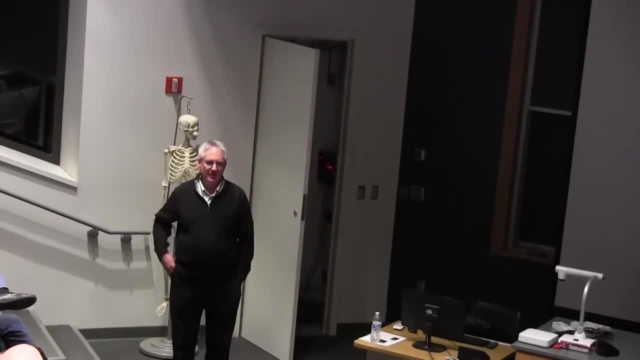 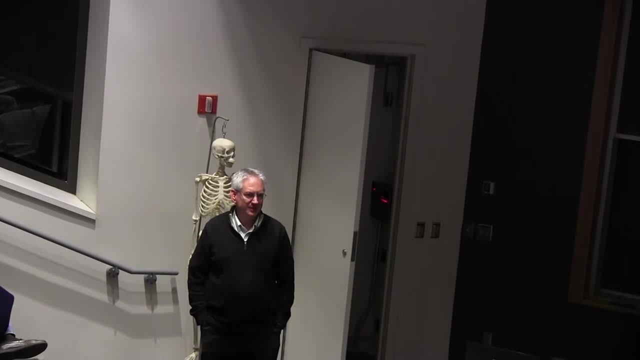 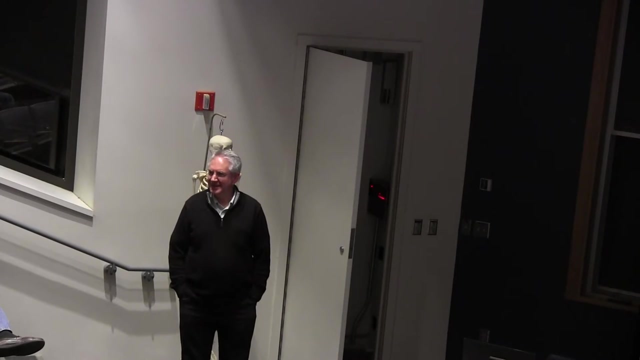 The campus looks completely different, although there are things that I recognize. Dinkman Sorenson was a new science building when I was here- Swanson, Swanson- But it's great to be back. So I'd like to talk to you about. 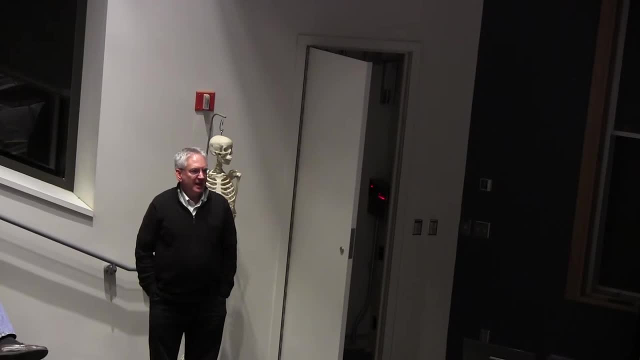 some of the things that I've done, And you can't say that you are the only person working on things. I've had an army of graduate students and undergraduate students helping me, And these are some of the current ones, And I'll point out Kate Pauls. 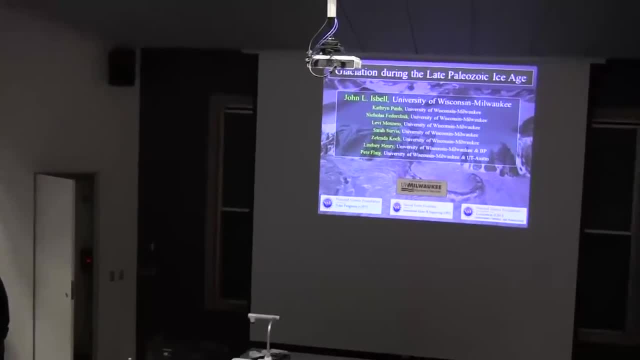 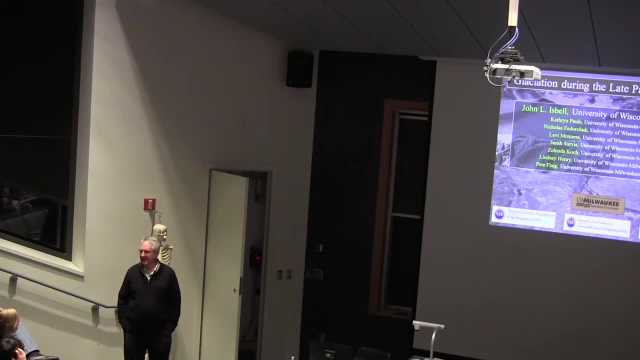 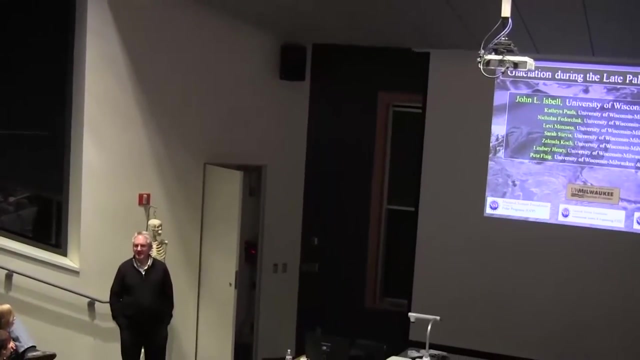 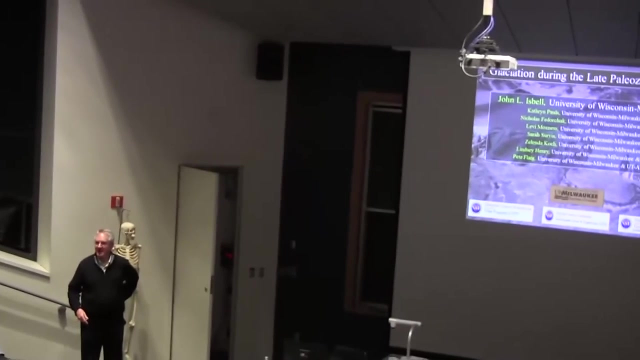 Kate's here tonight and she is an alum of Augustana College And three seasons in Argentina together. So you really can't do things without your graduate students. So these are my colleagues at the University of Wisconsin And just acknowledging funding support from the University, as well as various entities at the National Science Foundation. 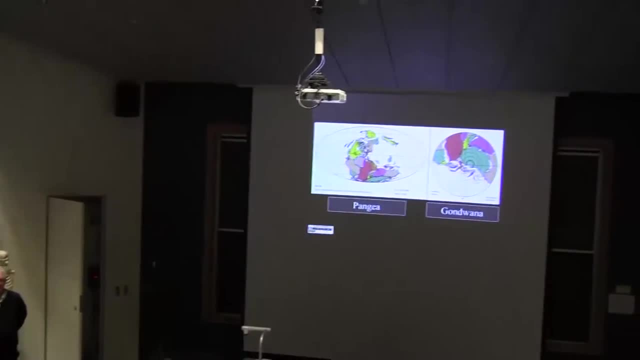 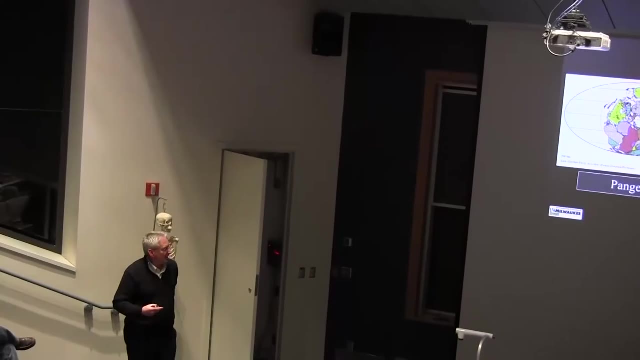 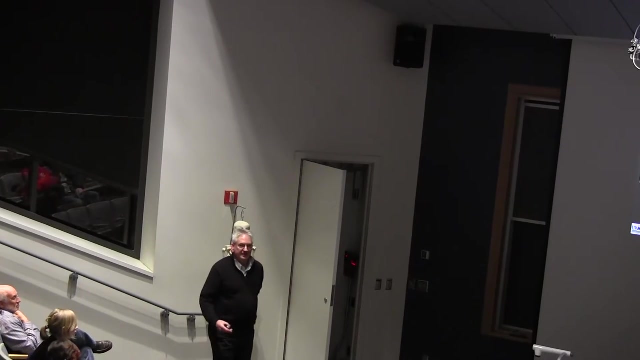 My interest is the late Paleozoic Ice Age and looking at it in terms of understanding deep time climate change And trying to understand some of the drivers that were going on and causing climate change and glaciation and then non-glacial periods 300 million years ago or so. 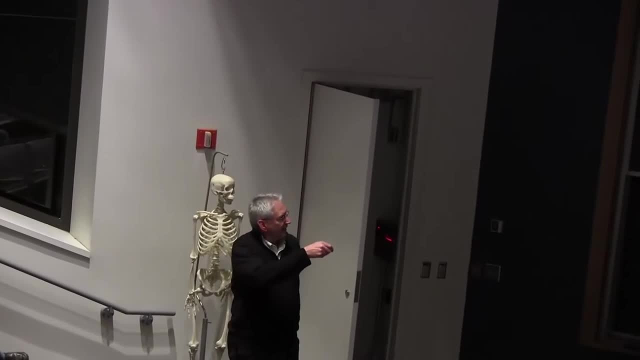 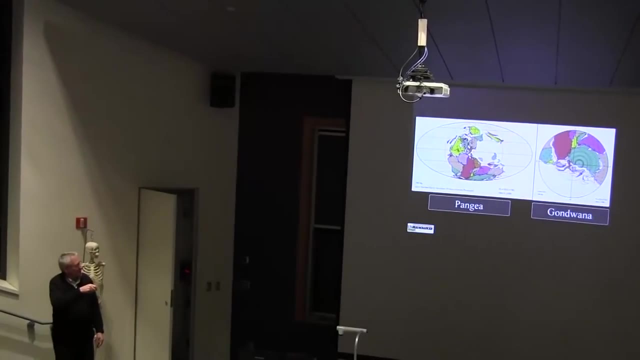 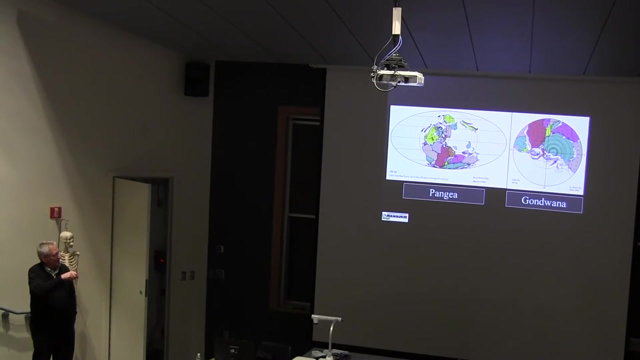 And at that time all the continents were together. You've got Pangea, which means all the continents In the Northern Hemisphere, Lower Asia And, my favorite, the Southern Hemisphere, Gaguana. So I'm going to be talking primarily about Gaguana. But I'll jump and just mention Siberia Just a little bit. And to understand the late Paleozoic Ice Age you really have to look at all the continents that were glaciated And it really helps then, by going from continent to continent, to be able to correlate and to understand how big the ice sheets were. 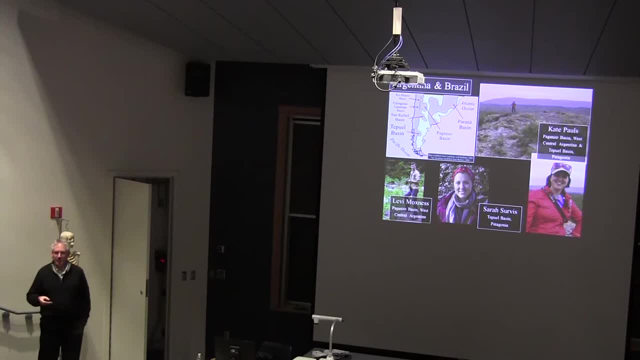 When did they disappear? Did they disappear at the same time everywhere? Was it diacronous across the continent? And then, of course, the students, And again I'll point out Kate, Who is currently a PhD student at UW-Milwaukee. 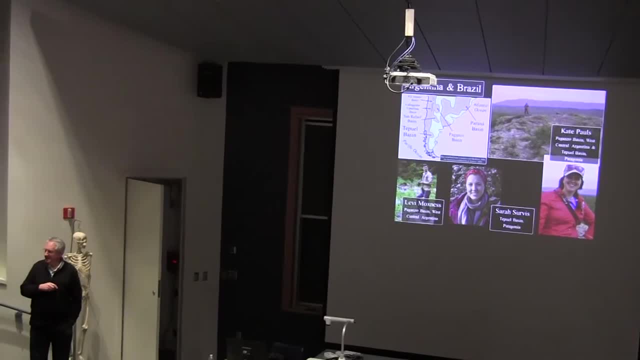 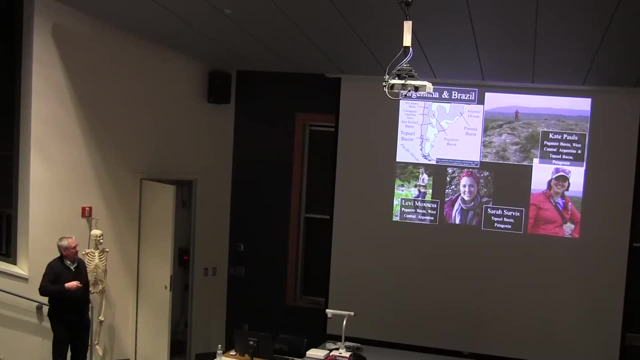 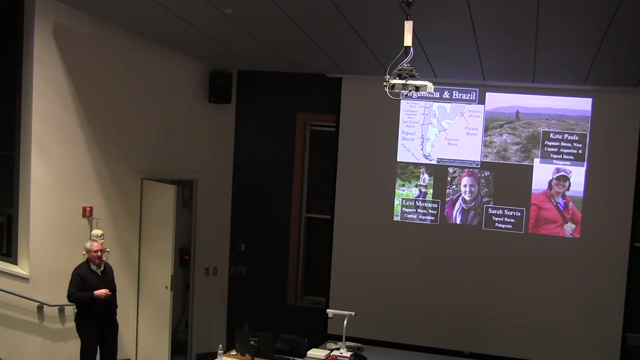 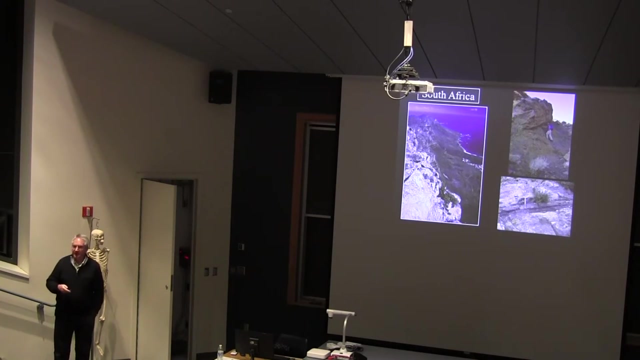 And graduated from here in 2011.. She's right here. So right now we've got projects going on in the Paraná Basin in Brazil And then various basins in Northern, Central and Southern Argentina, But I've also worked in South Africa trying to understand the glaciation there. 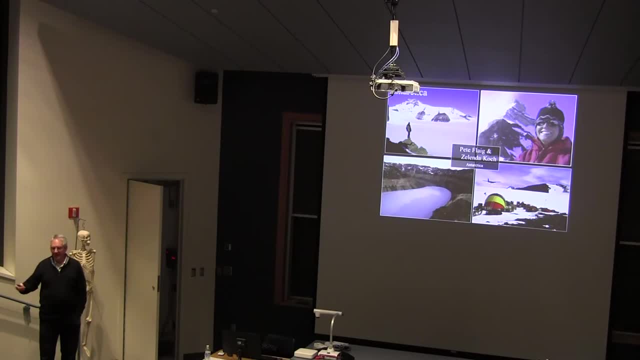 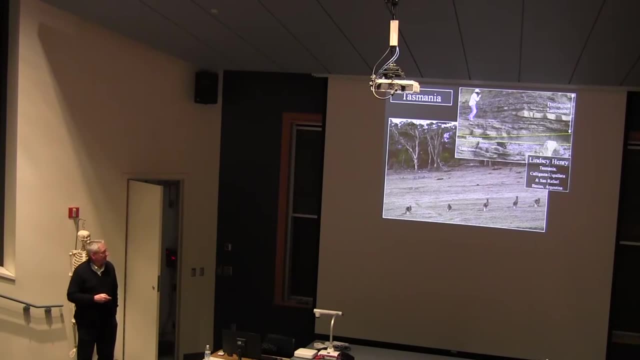 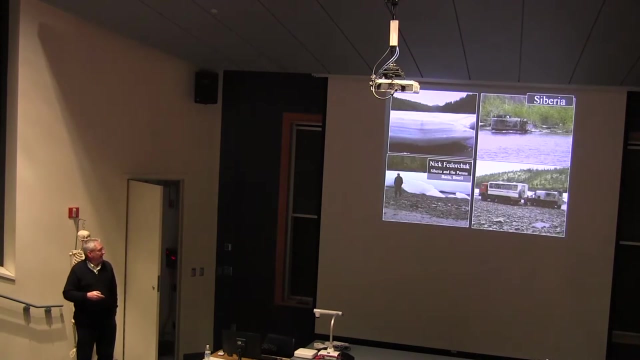 And obviously I spent a lot of time and camping next to Bill in the Antarctic And with students both grad and undergrad over the course of my career. Australia Photos of Tasmania, But also Western Australia, And it's thought that during that timeframe Earth was experiencing bipolar glaciation. 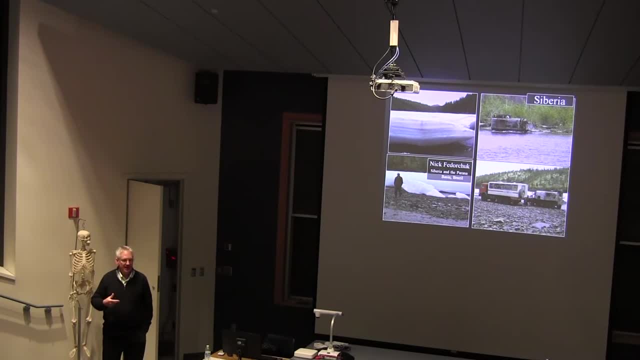 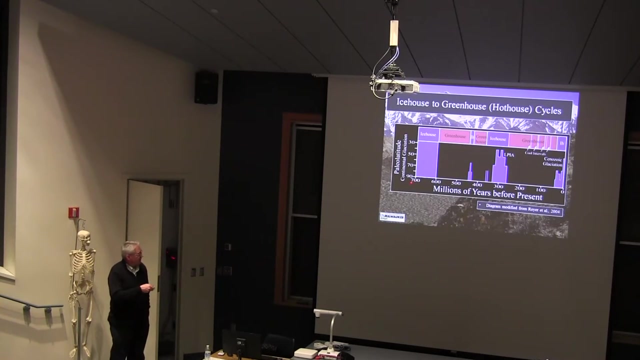 So if you want to understand the glacial history of the Earth at that time, You've got to go and look in the Northern Hemisphere as well. So I spent some time in Siberia looking at the deposits there. So this is a chart showing ice ages in Earth's history over the last 700 million years ago. 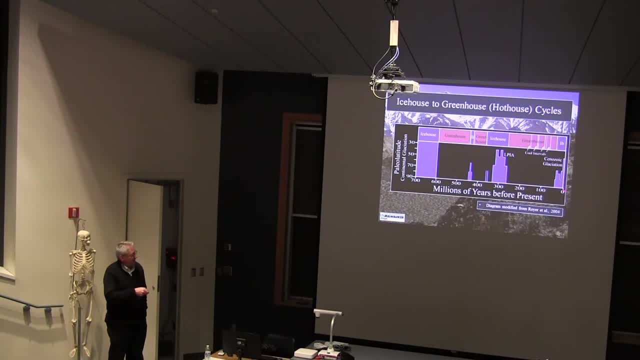 And here we are sitting at time zero, with years on this scale And then relative latitudes of the glaciers extended. So here we are sitting at time zero And wondering what's going to happen in the future. Well, we can't look and know for sure what's going to happen in the future. 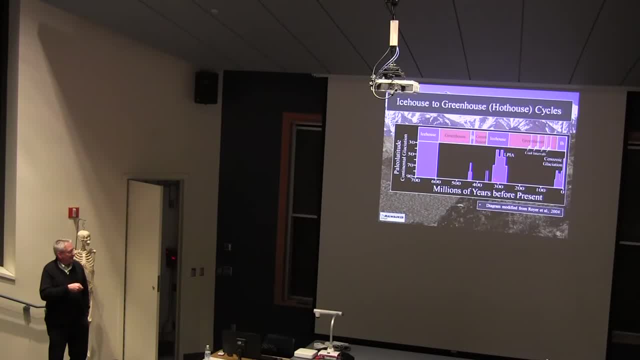 But we can look into the past And if we look into the past, around 300 million years ago, We have this major glaciation that's going on. It's known passionately as the Late Paleozoic Ice Age, And it has a couple of early blips. 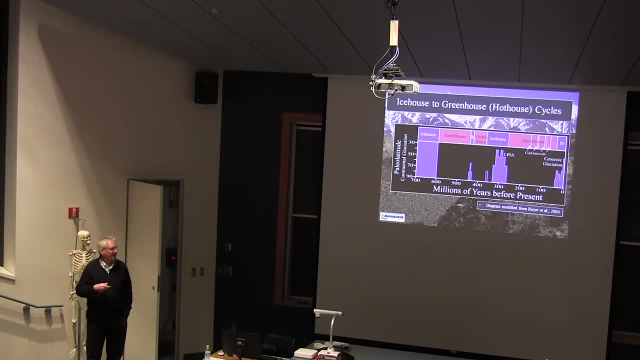 It gets well established during the Carboniferous And then ends in the Permian, And then Earth is relatively unglaciated, or at least in terms of ice sheets, Until we get to the Cenozoic Glaciation. So we're going to focus in on the Late Paleozoic Ice Age. 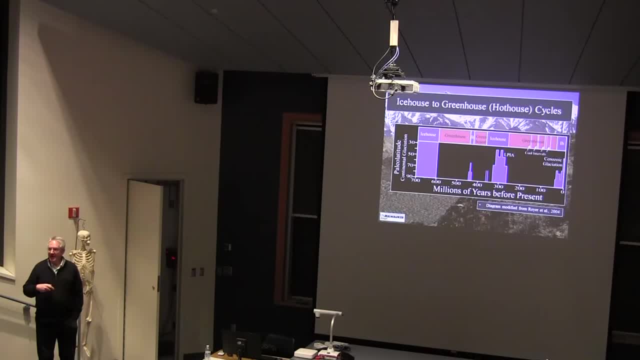 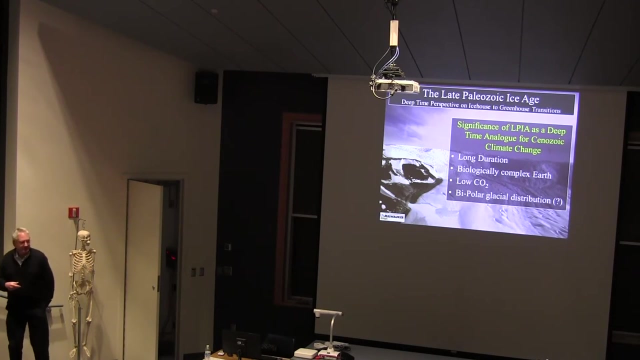 And that ice house conditions And then a little bit about its transition into a greenhouse Earth in the Permian. So the reasons why I'm interested in it and anyone is interested in it In part, is that it shares some similarities between the Cenozoic and the Late Paleozoic Ice Age. 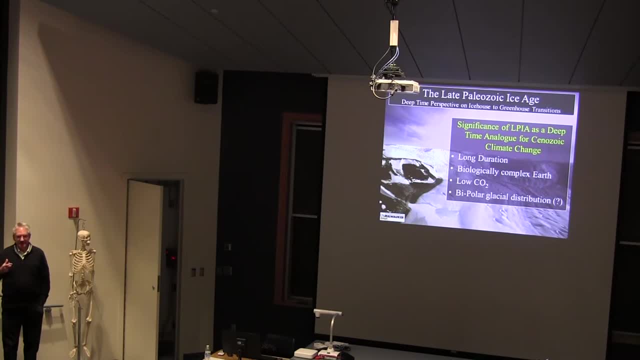 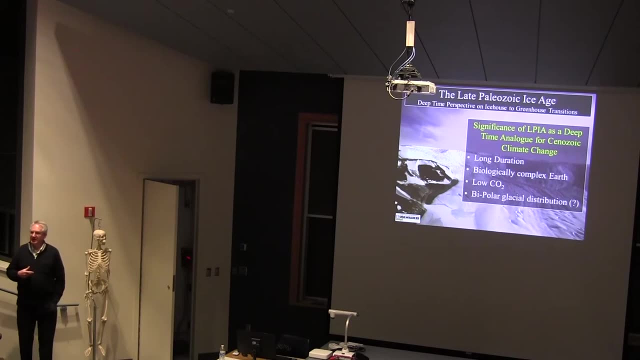 There are a lot of differences. The biggest difference, obviously, is that we had Pangaea. We had Pangaea back then and we don't today, But they're both long duration glaciations, Depending on whose time scale you use, whose age model. Sometimes, and if you use the Devonian, it's starting in the Devonian. The Late Paleozoic Ice Age can extend as long as 100 million years. Most people would put it somewhere between 60 and 80. But it really started. At least started to be glaciated during the latest Devonian. It's similar to the Earth today in that it's the only other timeframe that we've got a complex biota on Earth. No other timeframe, no other ice house has the same biologic history or complex history as the Cenozoic does. It's just these two: The Late Paleozoic Ice Age and the Late Paleozoic Ice Age, And the Cenozoic that has those. It's also a time when glaciation was occurring, when there was low carbon dioxide in the atmosphere. And a similarity is that people have thought that the Late Paleozoic Ice Age was bipolar like the Cenozoic Ice Age. But I put a big question mark here Because there hasn't been a lot of work done in the Northern Hemisphere. 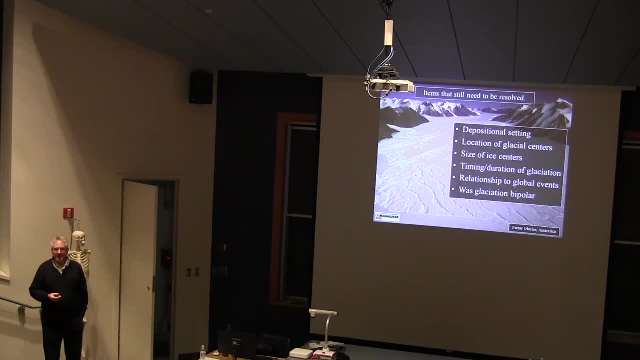 Okay, We know a lot about it. We've been studying the Late Paleozoic Ice Age for the last 90 years or so, But there's an awful lot that's not known, And these are the things that really are not very well established. 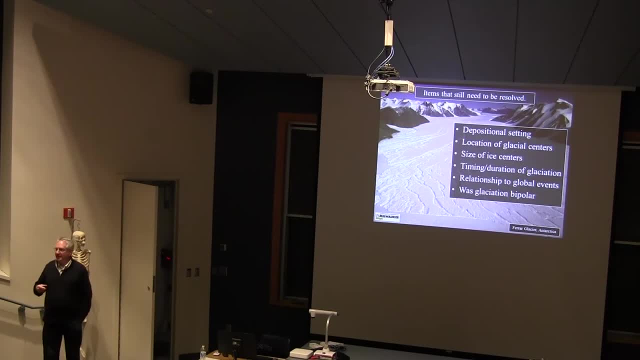 There's a lot of things we think we know And then the more we investigate it we realize we really don't know that much And a lot of what we thought we knew is wrong. So we don't understand the setting, The environments. 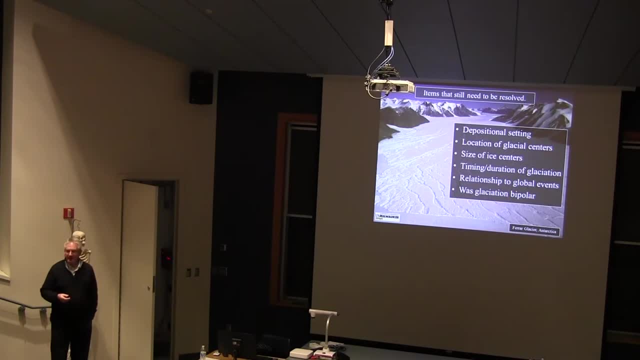 The environments in which the glaciation was occurring. We don't really have a very good handle on the ice centers, Although we're starting to get a better and better understanding of that. We don't know the timing very well In geology. to understand the history you really have to put a date on things. 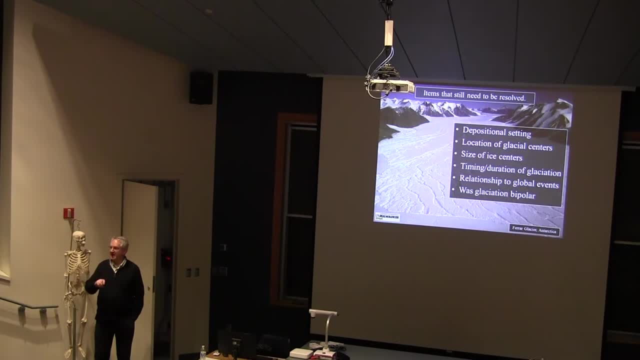 So that you can put it not only in space but in time And the Late Paleozoic Ice Age is really poorly constrained, And understanding how it relates to other global events. I grew up in West Central Illinois. I'm a first generation non-underground coal miner. 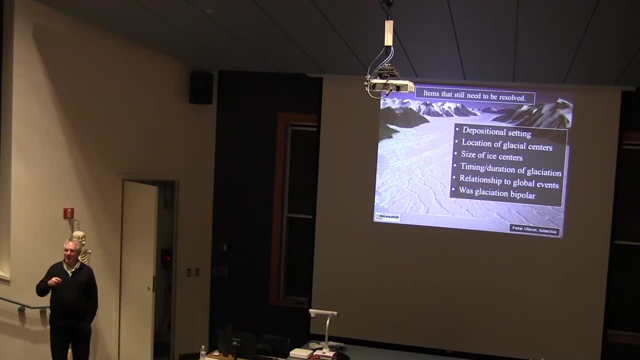 All my relatives were underground coal miners. That coal has been thought since the 1930s to be in part due to fluctuations in sea level, And those fluctuations in sea level are thought to have been driven by the waxing and waning of Gondwana glaciers. 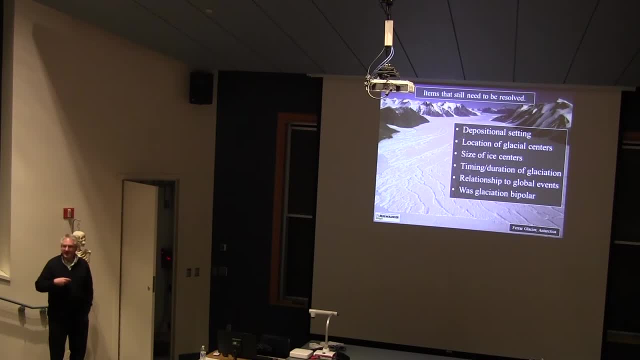 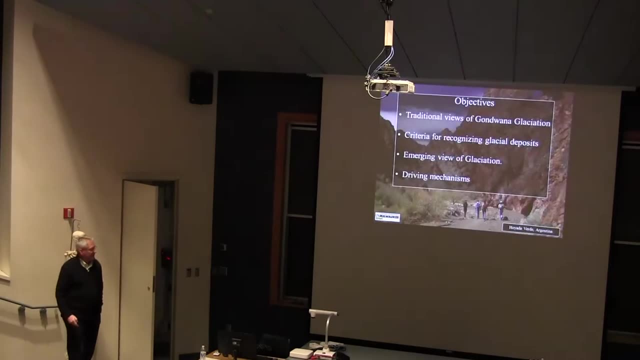 So We really need to get a better handle on how they're related. And then, finally, is it a bipolar glacial event at that time? So what I'd like to do tonight is just tell you a little bit about the traditional view. I'd like to spend an awful lot of time talking about some criteria in terms of identifying glaciation. 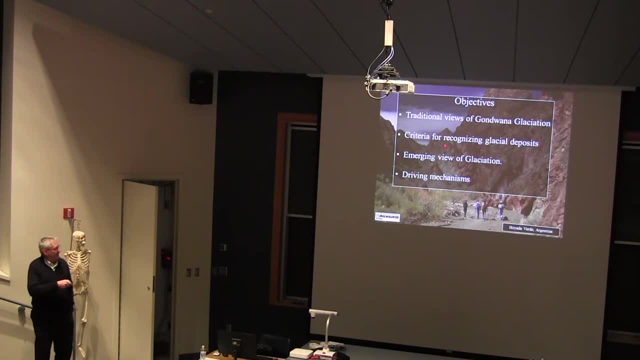 Why that's important, Telling you a little bit about our current view of the glaciation And then trying to address some of the things that was driving the fluctuations of the glaciers And the end of that ice age. So traditionally, we jumped to Gondwana. 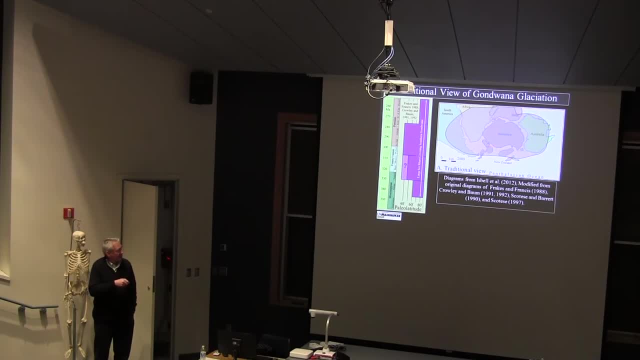 And we jumped initially to Dr Hammer and my favorite continent, Antarctica, Because at that time the South Pole was located. Well, it was actually located, and drifting across Antarctica In this fashion, and then off the continent, But Antarctica was centered over the South Pole. 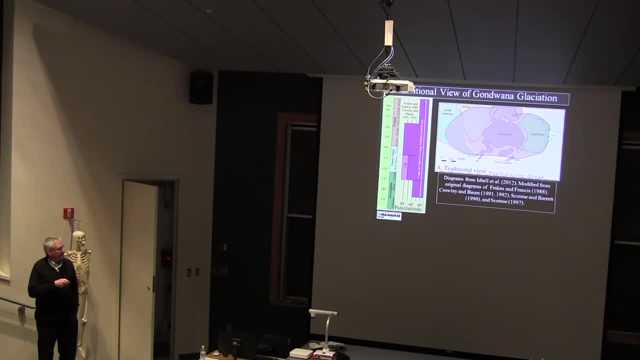 Over the South Polar Circle And it's thought that there was this massive ice sheet that extended outward from Antarctica And then it fluctuated and shrank and liberated water. as it shrank to the world ocean And sea level went up and down. 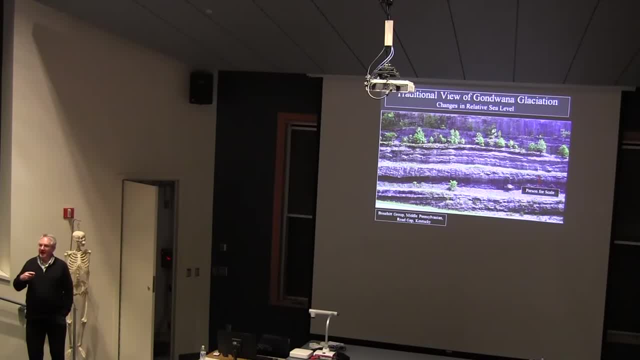 And so If we look at what's going on in this part of the world Instead of Antarctica, at least initially, What we see are cycles. This is from Pennsylvanian age rocks in Kentucky, And I pick it because it's a beautiful road cut. 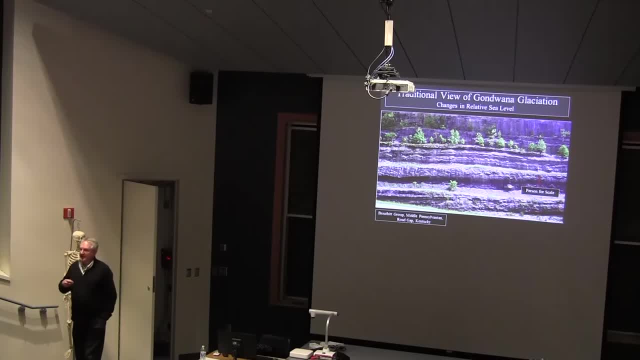 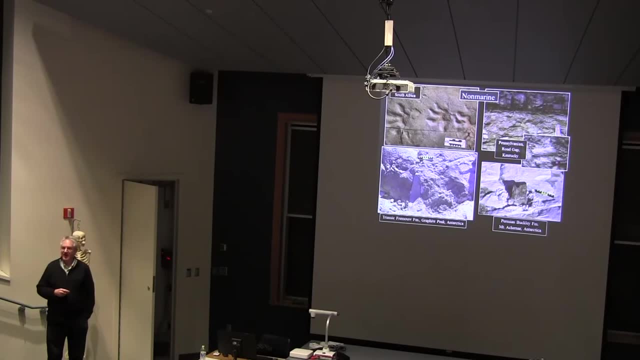 And you can start to see. If you start reading the rocks, You can see changes in sea level And the way that we would look at changes in sea level And your geology professors Would look at sea levels. We'd go out and we'd look at the strata. 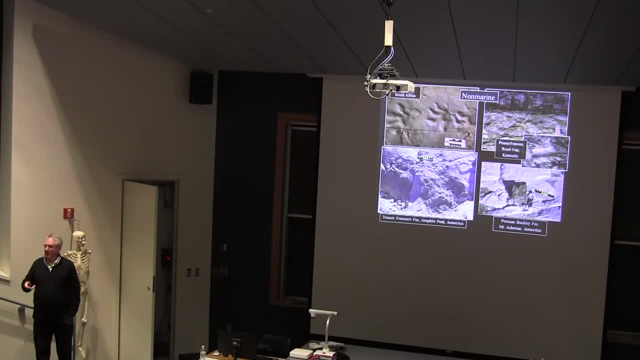 And we would progressively try to identify What rocks were deposited in a non-marine setting And the things that we would look for. We would look for evidence for organisms that live on land. So in this case this is from South Africa: Some vertebrate footprints. 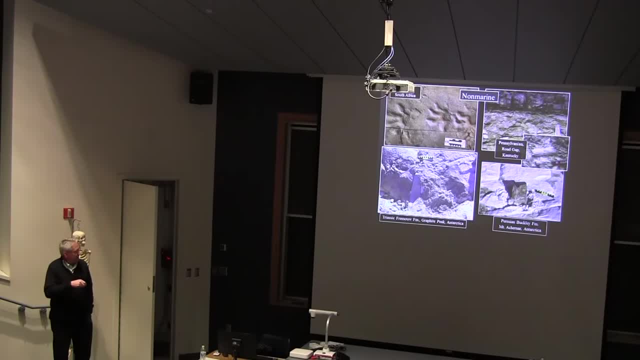 This is from one of Dr Hammer's site On graphite peak Lystrosaurus. maybe Here you can see the rifts. Here are some vertebrates. So if you see non-marine animals, You know you're sitting in a non-marine setting. 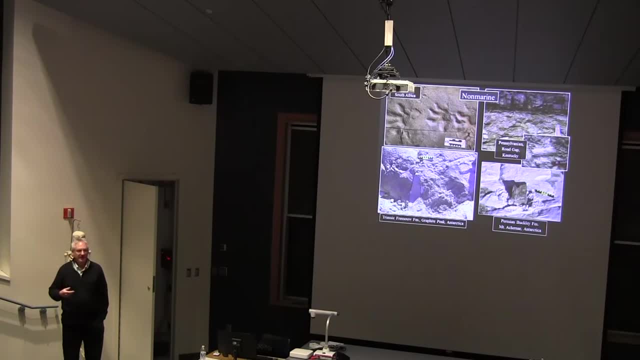 If you see coal, Coal forms on land. It may be wetlands, But it forms on land. This little thing here is a root. These things are root hairs extending out. Here is Another root. This is the root of the Lepidodendron tree. 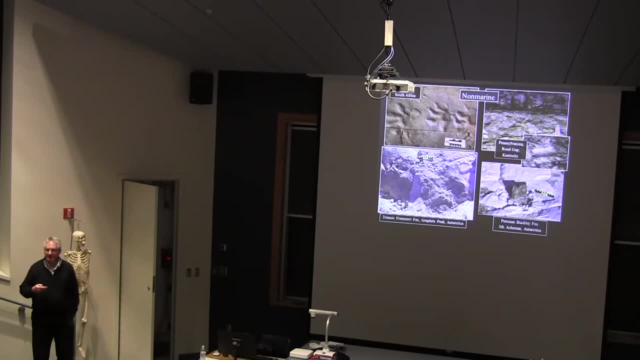 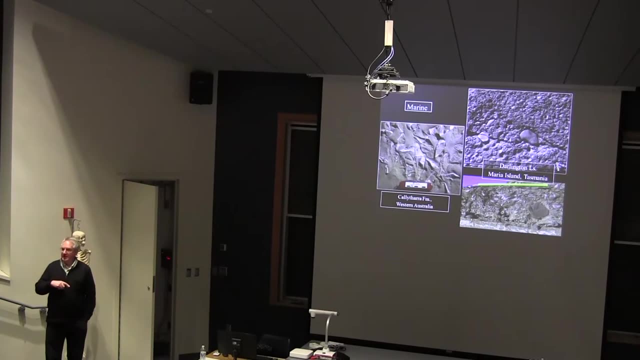 Here is Amartica And here is a stump in a fossil forest. So if you see these things, You can identify the rock units as being non-marine Versus if you start seeing marine fossils. So here are some brachypods. 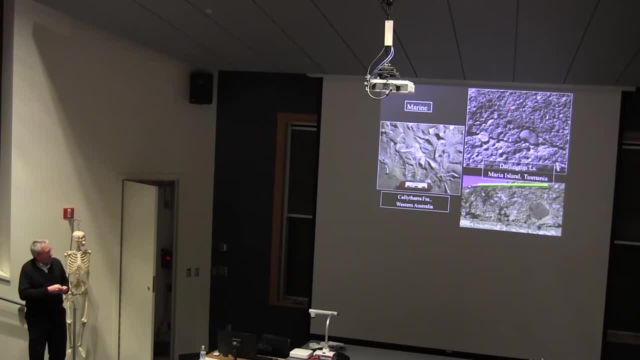 And this is in Western Australia. All these knobby little things over here Are A bivalve clam- It's about the size of my fist- Called iridesma, And then down here You can see the shells, And these are iridesma. 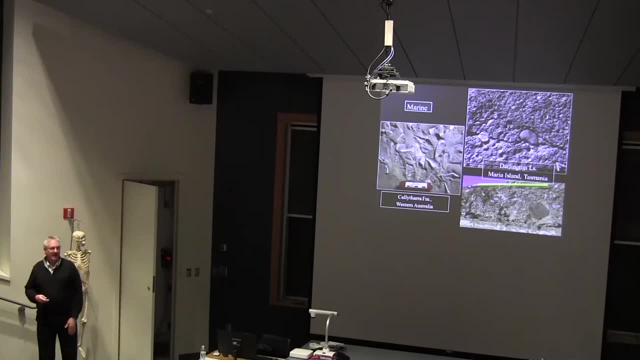 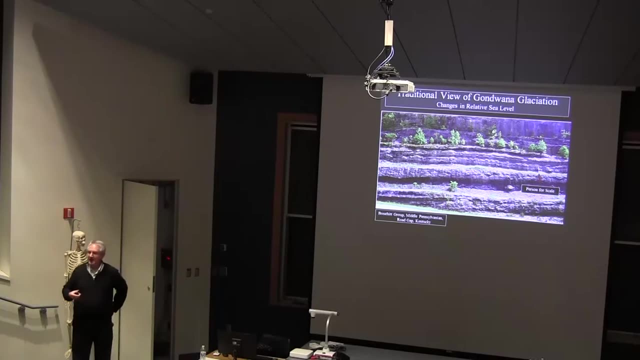 As well, And there's some pectin, But it's telling you you're in a marine setting, So You can go out And you can go through These units, And you can go layer By layer By layer. 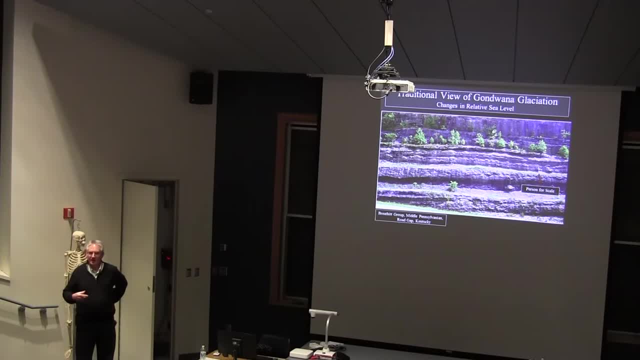 And you can identify Whether they were deposited In a non-marine setting Or in a marine setting. And when you do that For the strata Of the Pennsylvanian age In North America, You see this alternation. 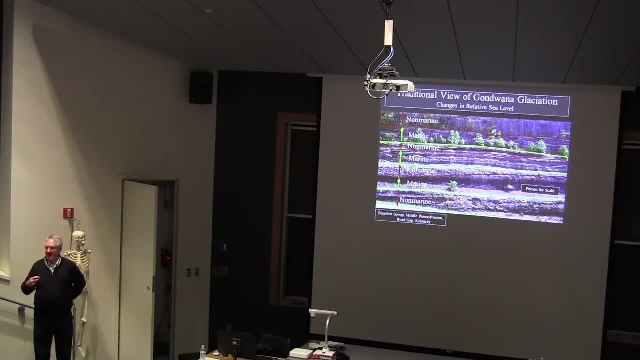 Between non-marine And marine, Telling you That either the land surface Is bobbing up and down Or The sea level Is rising And falling Through time. And If it's rising And falling, Then you need a mechanism. 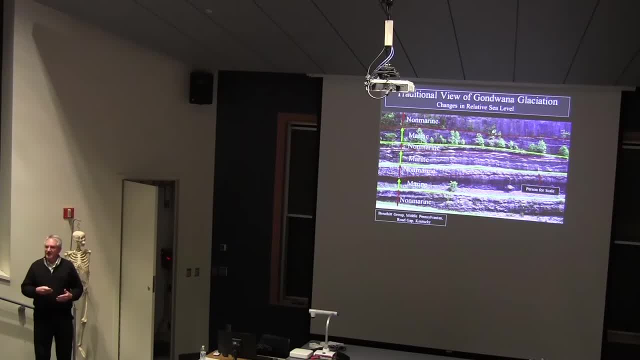 To produce that And that mechanism Back in the 1930s, A guy named Harold Wanless And Shepard From the University Of Illinois. He was One of the first People To produce Iridesma. 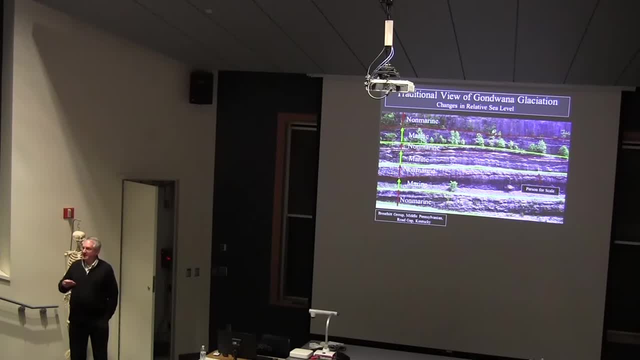 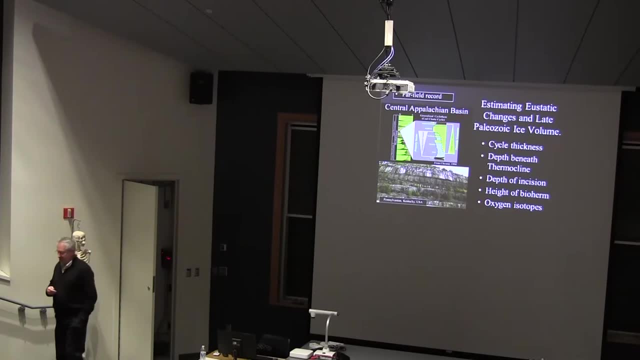 And In the University Of Illinois Attributed that To the waxing And waning Of glaciers In Gondwana. And Since then There's been a lot Of work That's been done. 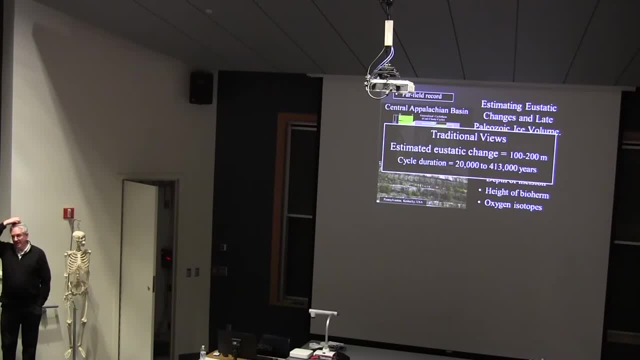 On the cyclothems And the coal bearing units And What they Have identified Is That traditionally That- And that view Is changing- Traditionally It's been thought That They represent Between a hundred. 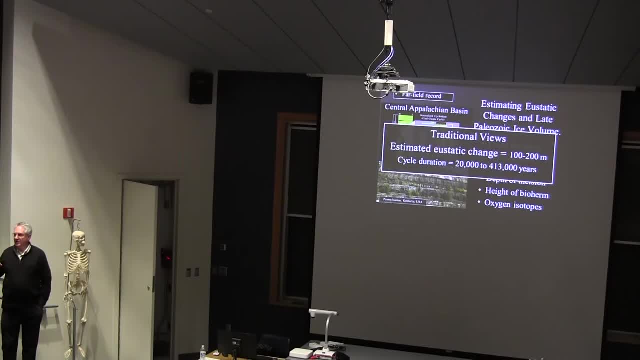 And two hundred meters Changes In sea level, And we now know That that number Is much, Much lower. But that's What the traditional View was And that was One of the things That drove The modeling. 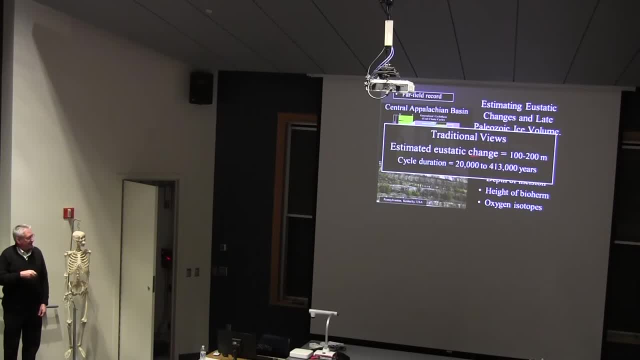 Of this Huge Ice sheet Centered Over Antarctica, And that those cycles Had a duration, Where they alternated From marine And non-marine, Of twenty thousand To four hundred And thirteen thousand Years, Which are 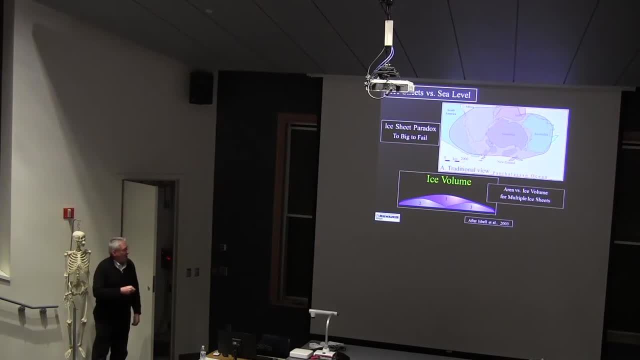 In the Range Of Orbital And that Has given us This view Of this Immense Ice sheet, Because this Is the size Of an ice sheet On Guana That you need To be able. 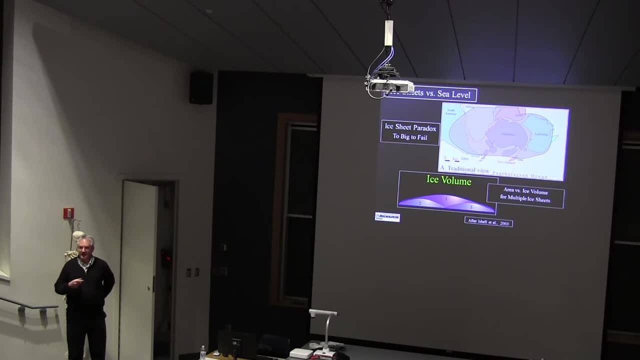 To have Two hundred meters Changes In sea level, But there are Some big Problems. It's really Difficult To get an ice sheet Of this size Centered Over Antarctica To get the moisture To be able. To grow An ice sheet Of this size. They become Incredibly Stable. They don't Fluctuate. So Instead of having A big Ice sheet, That's really Stable If you want Fluctuations. To go on. You need To have Smaller Ice sheets That are more Sensitive To changes In Global Temperature, But If you have Smaller Ice sheets, That may Be A good. 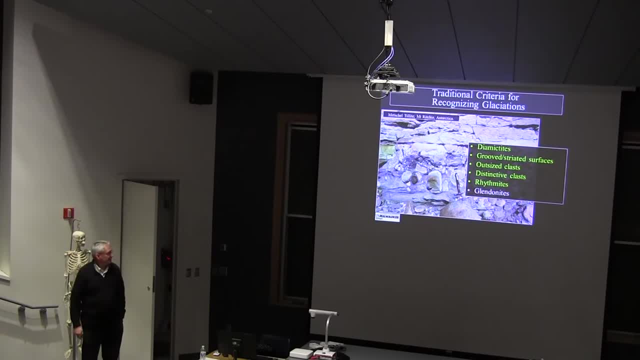 Thing To Get A Ice Sheet. So Let Me Tell You About Why They Were Originally Identified To Be These Big Ice Sheets, And The Criteria. 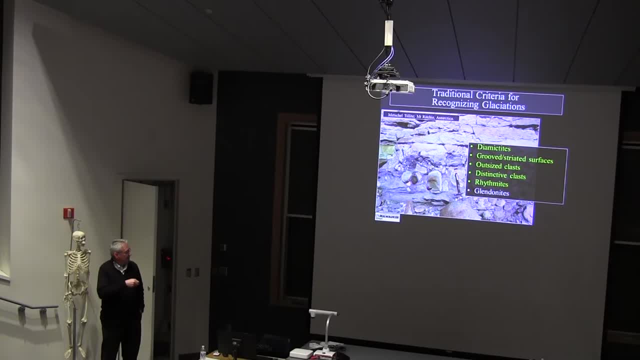 So Dynictites Are These Poorly Sorted Deposits That have Large Clast In Them. They Have Sand, They Have Clay, So It Just Is Jumble. 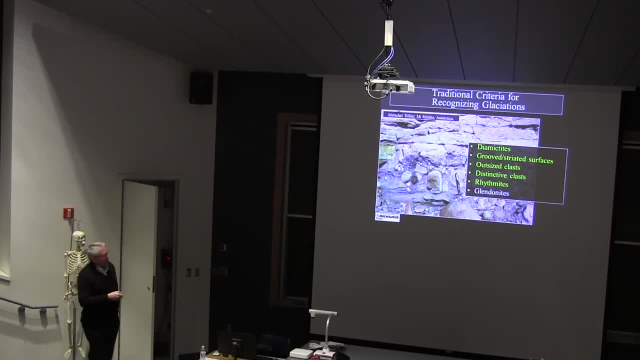 Of Deposits And Those Deposits Glaciers, Typically Deposit In Icebergs, Distinctive Class Flakes And And Erosional Features, Rhythmites, Bars. 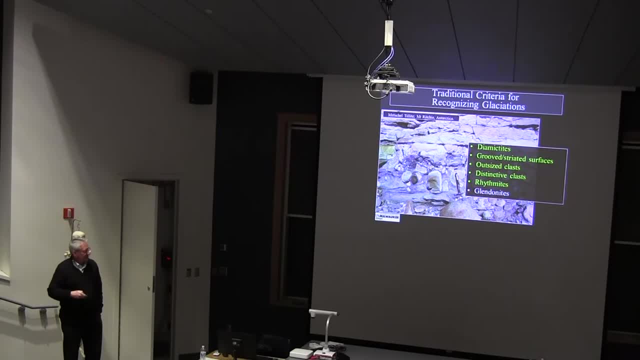 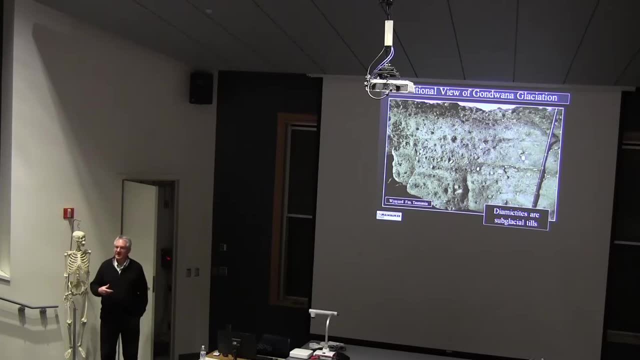 If You've Ever Heard The Term Bars- And I Won't Talk About Glendonites, But There's A Whole Slew Of Glacier Tills And 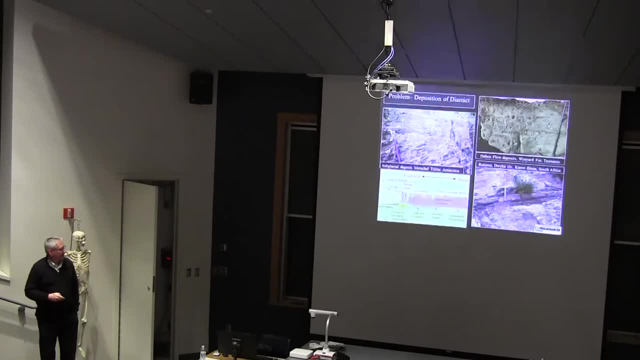 So You Draw A Ring Around It If There Was A Glacier Over This Area. The Only Problem Is Is There Are A Lot Of Other. 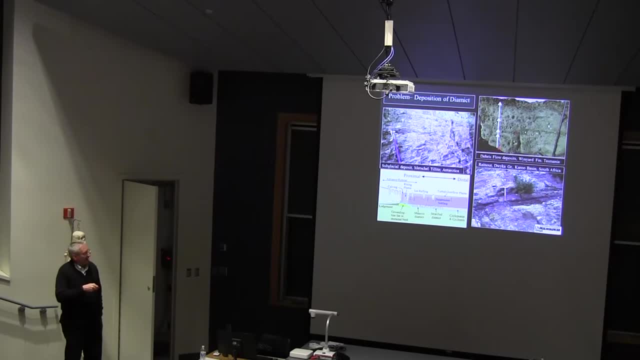 Things That Are Being Bedded, And It's More Characteristic Of Mud Flows, Debris Flows That May Or May Not Have Anything To Do. 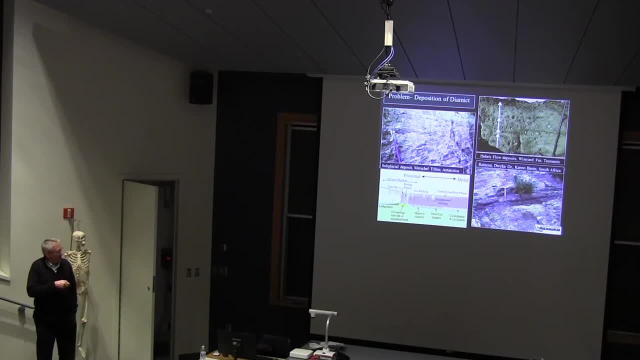 With Glacial Deposits. So If We Strip The Water Rises To The Top Is Carrying Suspended Material That Extends Out Into The Ocean. 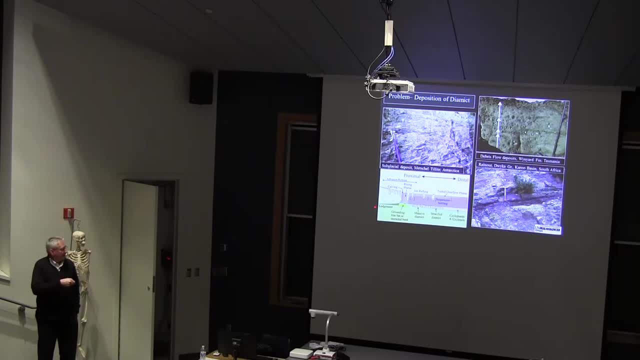 And The Fine Grain Material Rains To The Bottom And Ice Birds Then Carry Out To The Sub Glacial. Not, You've Got Glaciers. 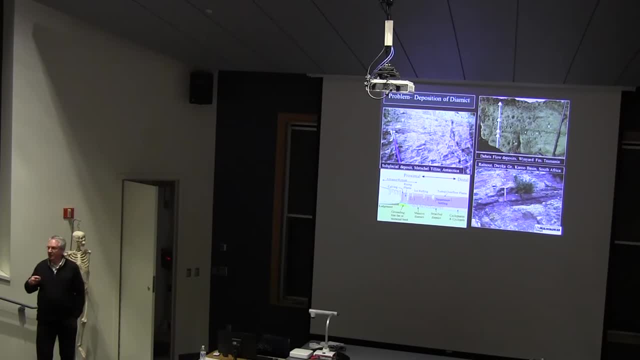 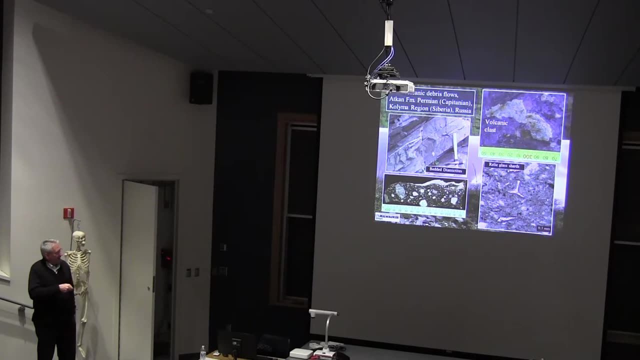 Everywhere All The Time, At The Equator, At Sea Level Today, And That Gives You A False Impression Of The Size Of Glaciers. But 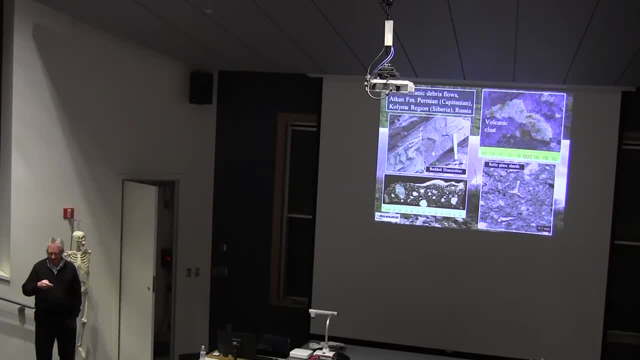 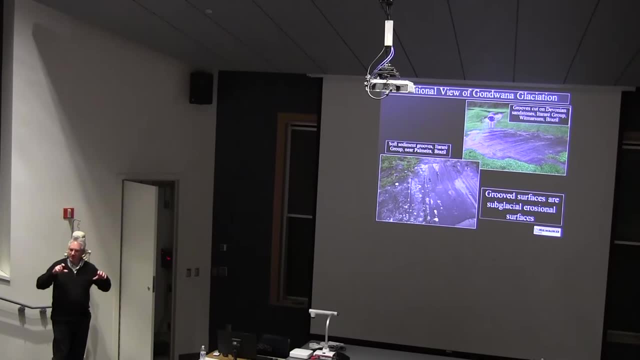 They're Dymectites And They Have Been Interpreted In The Past To Be Sub Glacial Deposits, Grooved Surfaces Where It's Thought. 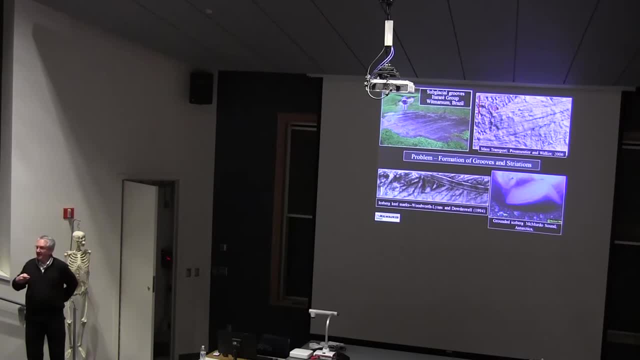 That The Glacier Would Move Over In. But There Are Other Things. If You Have Large Slide Blocks That Slide Down A Continental Slope At 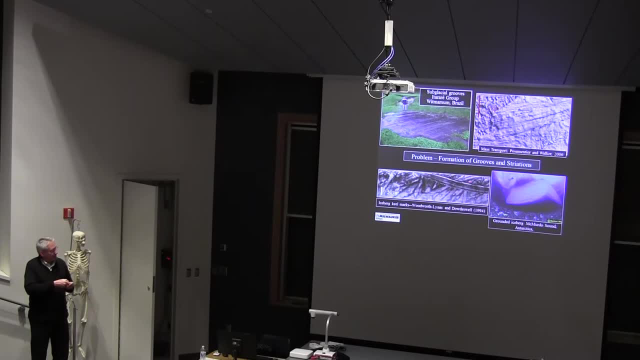 Any Latitude, They Produce A Grooved Surface. If You Have Icebergs In The Southern Hemisphere- I Think There Have Been Icebergs That Have- 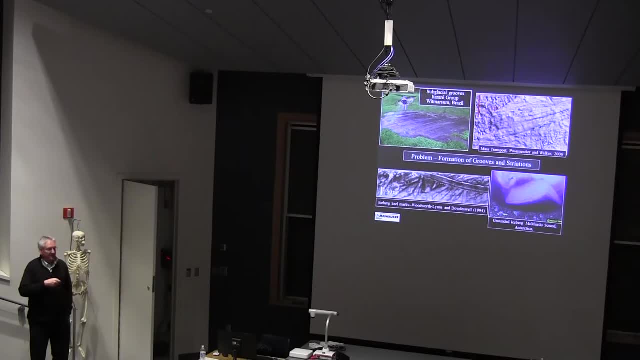 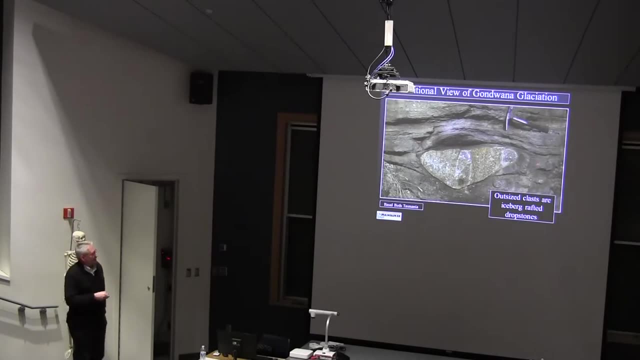 Extended Off The Coast Of North Carolina In The Recent Past. There's No Glacier Near North Carolina. Iceberg Melts And Accumulates Material On Its. 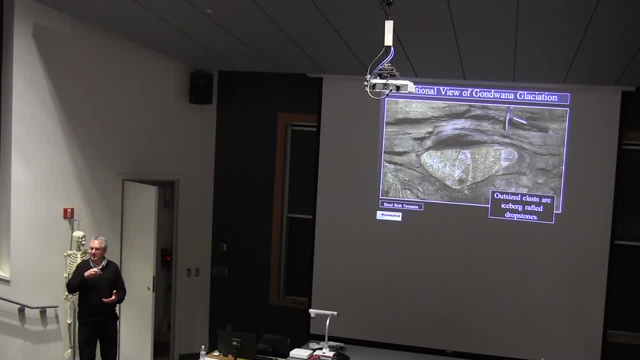 Surface, Or It Melt Out From The Bottom And On The Surface. When It Rolls Over, It Dumps Coarse Material Into Environments. To That. 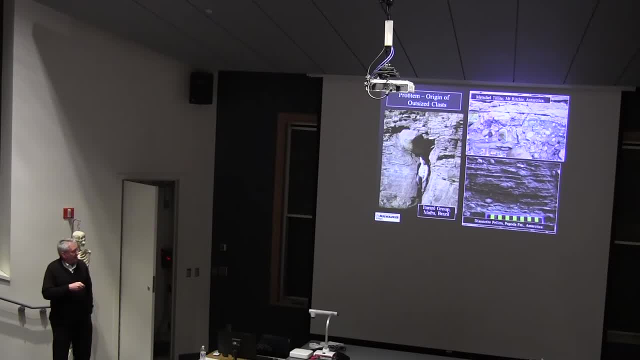 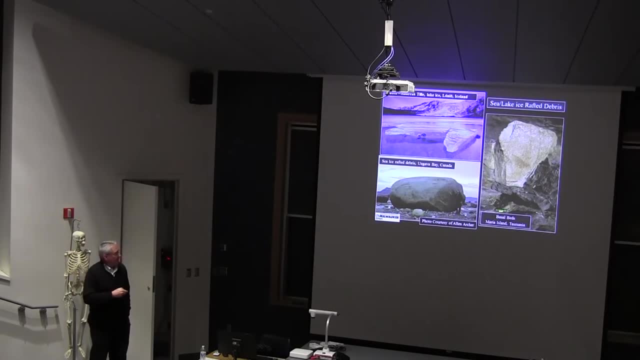 And Here's One In Brazil. It's Piercing Strata, And All Of These Are Probably The Result Of Iceberg Activity, But Sea Ice Transports. 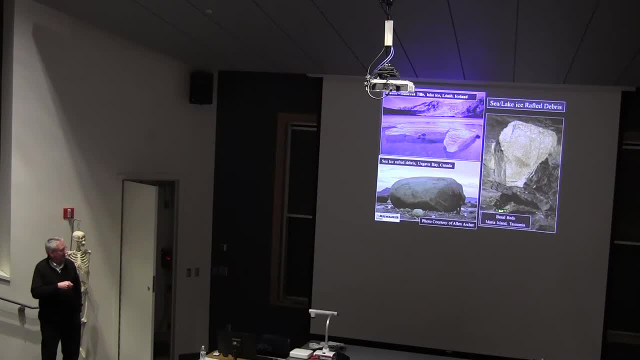 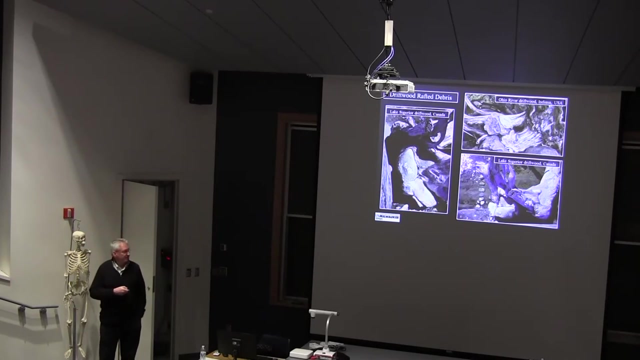 Material And Lake Ice Transports Material. Sea Ice Can Pick Up Things That Are As Much As Six Tons In Terms Of Weight, And They 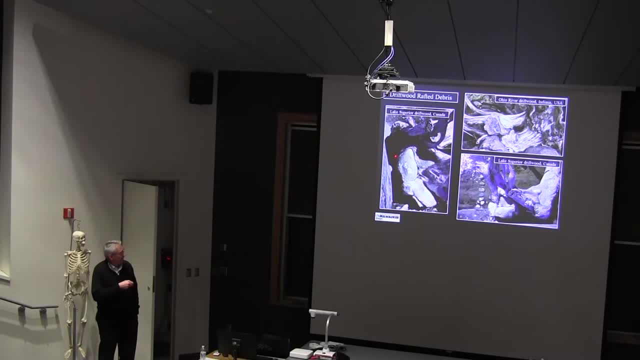 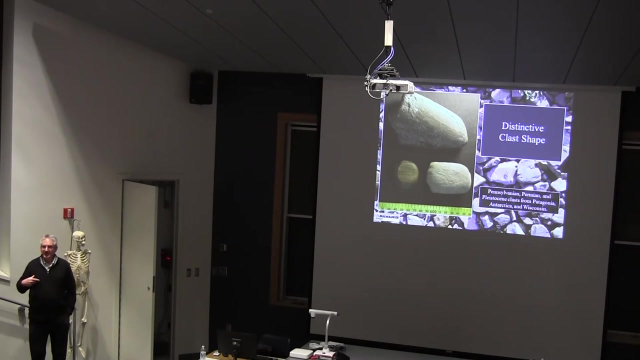 Can Transport Composite Material And This Boulder We Interpret To The River. They Will Transport Material And Drop Things In, So You Have To Be Somewhat. 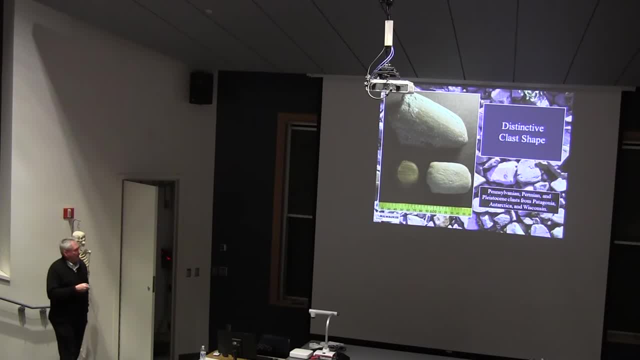 Careful In What Dropped In. If You Close To A Volcanic Center, Hummus With Scratches On, And Those Are Distinctive Of Being. 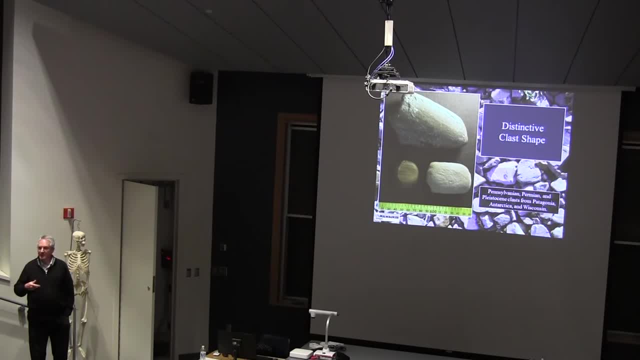 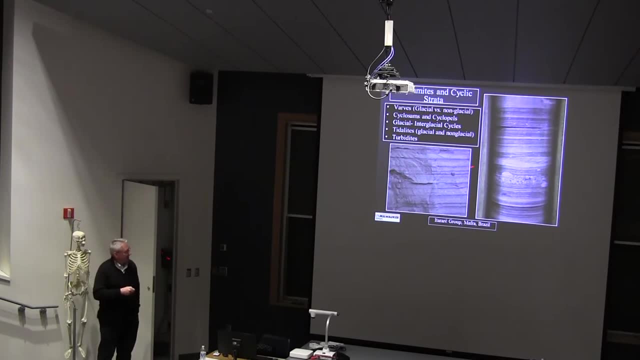 Glacial. So If You Can Identify Those Class As Drop Stones Or Within A Subglacial Environment That We Think Subglacial In The Input, 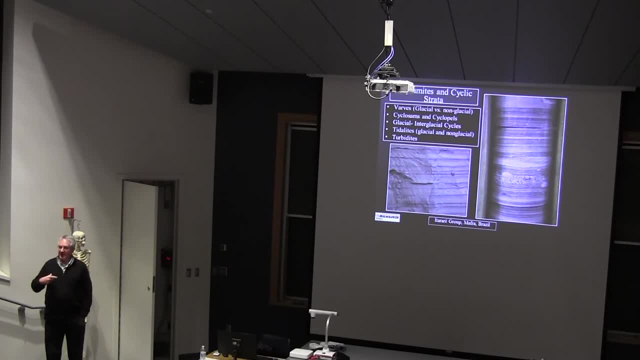 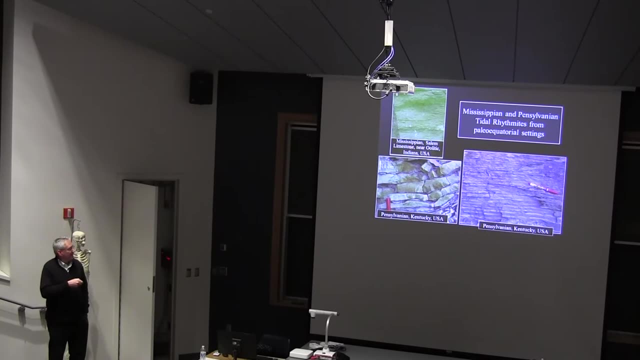 And Then The Turnover Of Lakes And They're In The Rock Record Used As Strong Evidence Of Glaciation. However, You Get Rhythmites In. 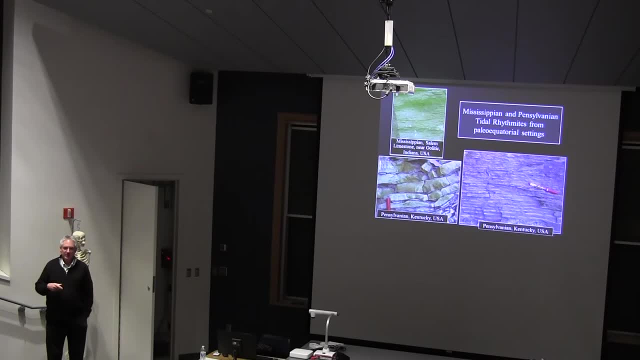 Limestones That Were Deposited Out To Wyoming Hill And Look At The Rocks Just Outside Of Muscatine. They're Beautiful Laminated Silts. 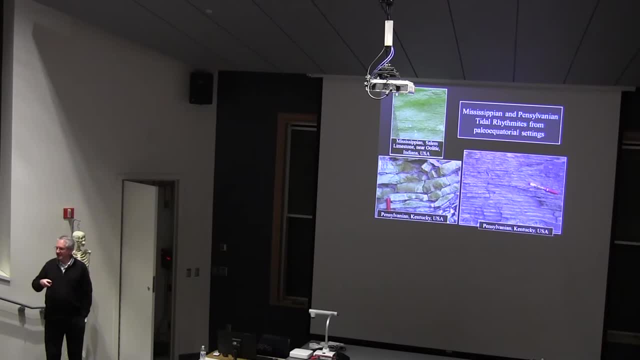 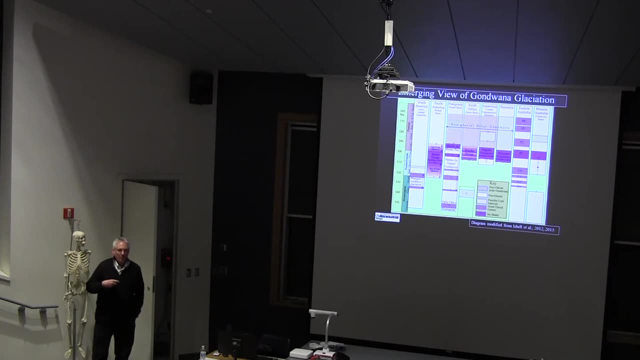 And Clays And They're Probably The Result Of Tidal. They're Not The Result. Really, Scrutinizing What The Record Is What We Find. 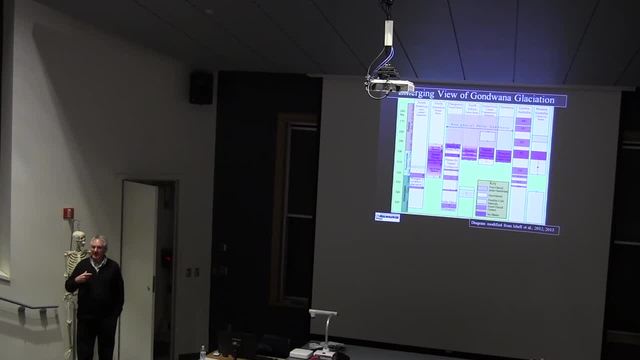 Is, We Don't Have This Extensive, Continuous Glaciation Of Really Large Glaciers. But The Record Breaks Down So It Changes From Work. 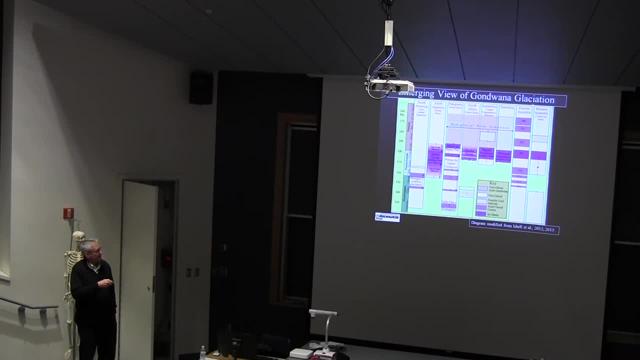 In Patagonia And South Africa, Antarctica Going Over To Tasmania In Australia, Eastern Australia And Western Australia. The Glaciation Was Not Continuous, So Here's. 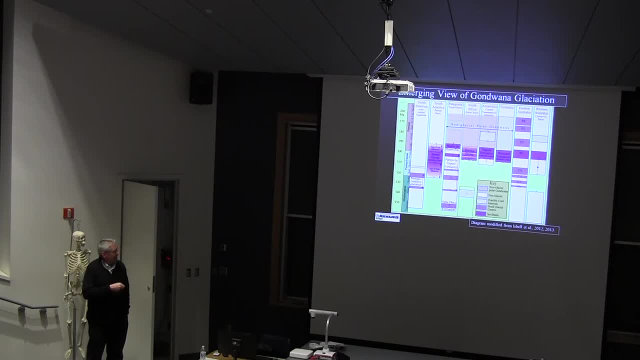 Our Time Scale Going In South America, While They're Not Occurring Elsewhere. Sometimes They're Occurring In Australia And They're Not Occurring In. 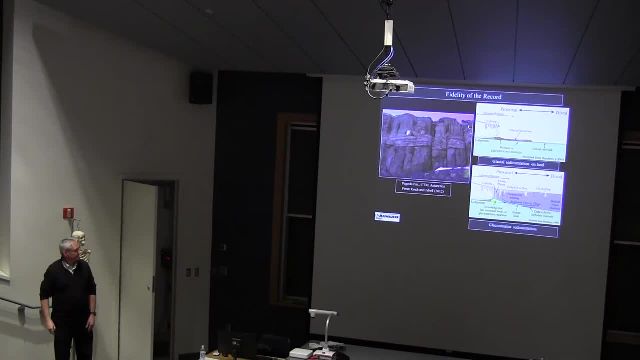 Antarctica, Or In South Africa, South America. So The Record Is Here. There's This Concept That, As A Glacier Advances, It's Eroding And Destroying. 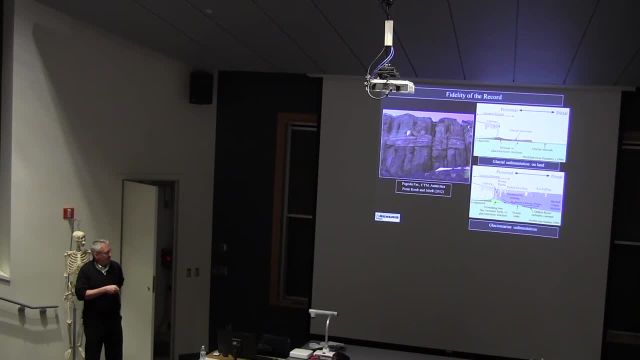 Its Entire Record And It Does Tremendous Amounts Of Erosion. But When You Get Out In The World Of Settlement While Preserved Near 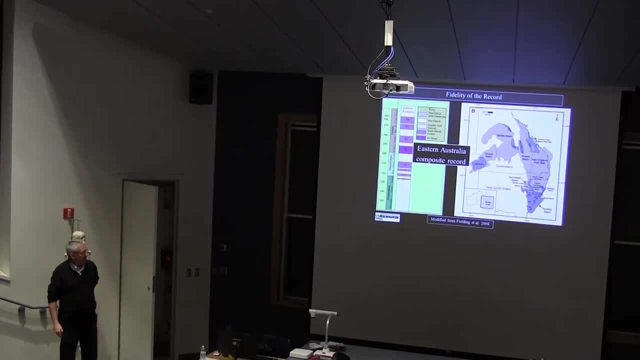 Continuous Record. Even Though Sedimentation May Be Slough, There's Very Little Erosion At Least Glacier Resulting Erosion When We Look At. 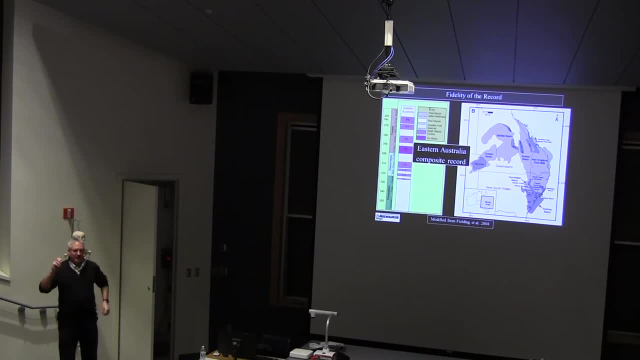 The part of the record is from down here and you're hopscotching around. It'd be like looking at stuff in the Appalachians, looking at stuff in Illinois, running down to New Mexico, and coming up with a record for North America. It looks great, but you've 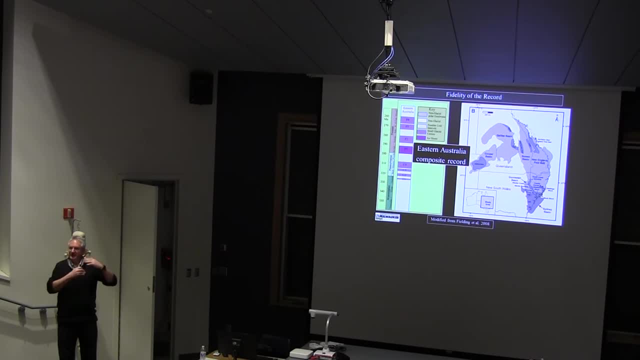 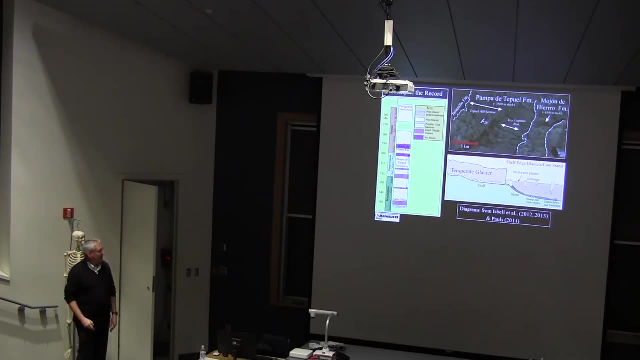 only got a few meters of strata in any one place and you're piecing it together So it looks really good. but there's a lot of problems if you're using these composite records One place, and why Kate and I are so. 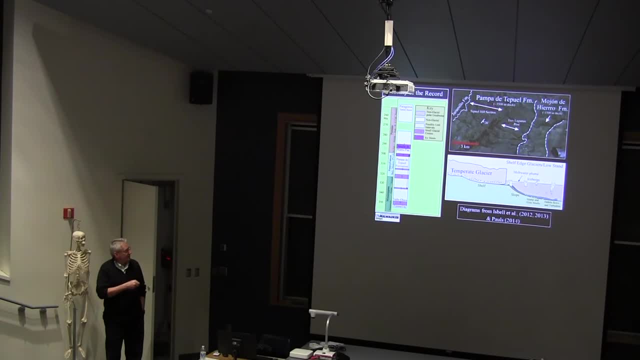 interested in Patagonia is that this is one of Kate's sections that she was working on for her master's degree. The strata are dipping there and they run from the Mississippian up into the Permian and you have 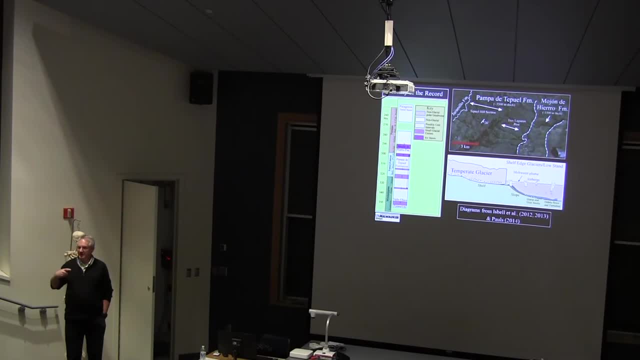 5,000 meters of continuous section So you can walk through it. You can start down here and start in the Mississippian and you can walk all the way through and it's a glacial marine section and you have an almost near-continuous deposition. that went on. 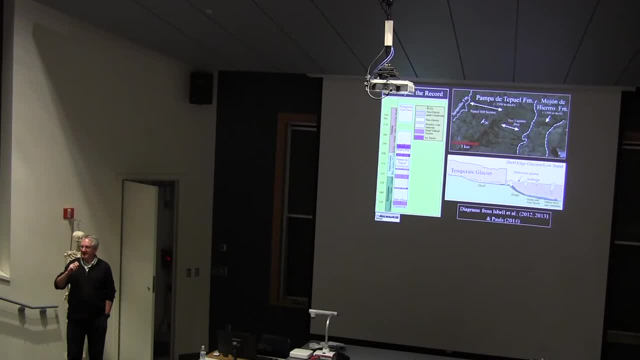 The only big problem is dating it exactly, and that's a real big problem there. It's a beautiful record, but the control on time. we can put a gross estimate on when things happen, but we can't put the exact date on that. 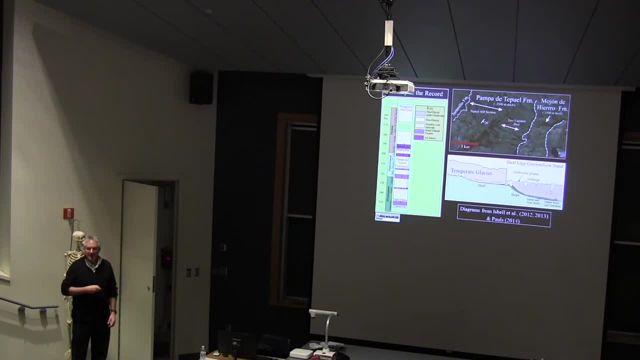 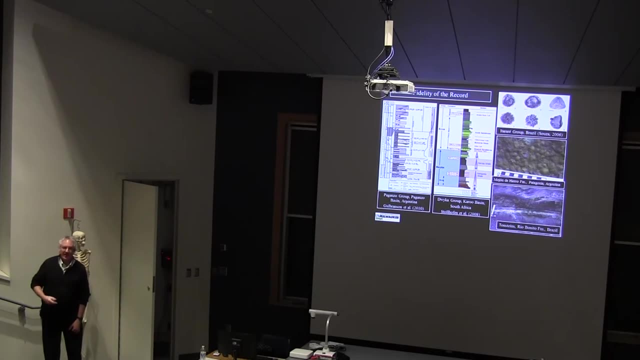 The glaciers there made it out to the continental shelf and then poured material into a deep water basin. So it's a beautiful record. There are other areas that we're just now starting to see good radiometric dates. Mostly the record in Gatawana is correlated, based on 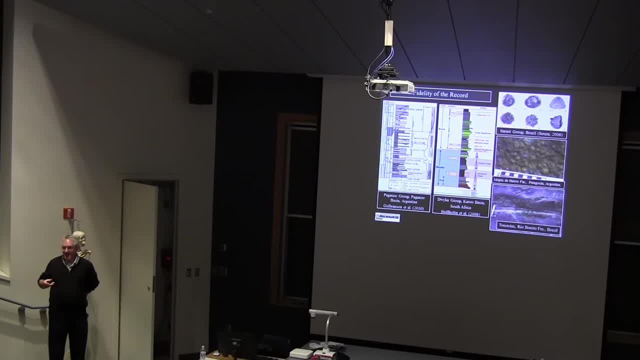 pollen and spores, and that's great, but it's really inaccurate, So we need something that's better. In Argentina, a lot of correlation has been done not only by looking at pollen and spores, but looking at invertebrate fossils, And that's good, but everything is endemming to South America, So you can date it. 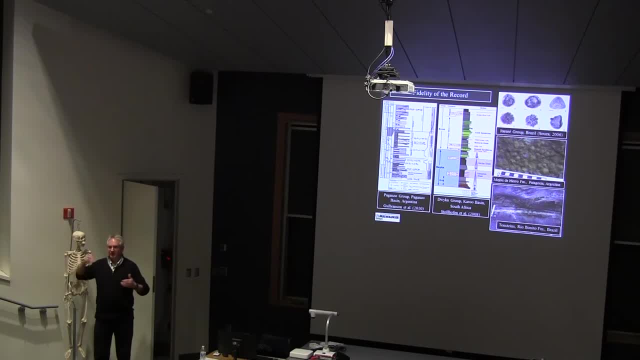 within a basin and correlate it within a basin, but it's difficult to do it from one place to another. But what we're now starting to find is we're starting to find a lot of volcanic ash, and especially in Brazil, And that's why Brazil is so interesting to us right now, because we can date the rocks there. 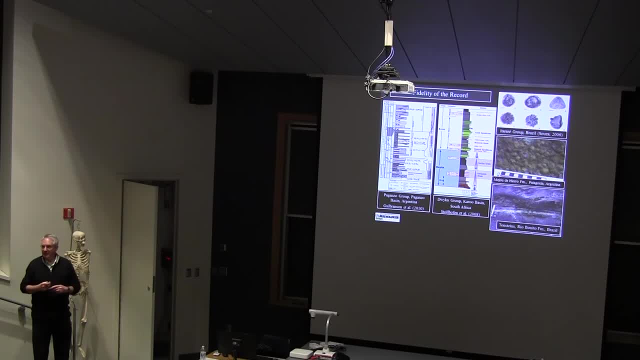 And we found that in western Argentina- not in Patagonia, but northwestern Argentina- there's a lot of volcanic ash. In South Africa there's a lot of volcanic ash. So it's starting to develop and that record is getting better and better through time. So let's take a tour then of this glaciation. So glaciation really begins before this chart. There's a couple of blips in the Devonian just before I start this chart And that's kind of start stop. But the main glaciation of the late Paleozoic Ice Age starts in South America and it starts at about 335 million years ago. 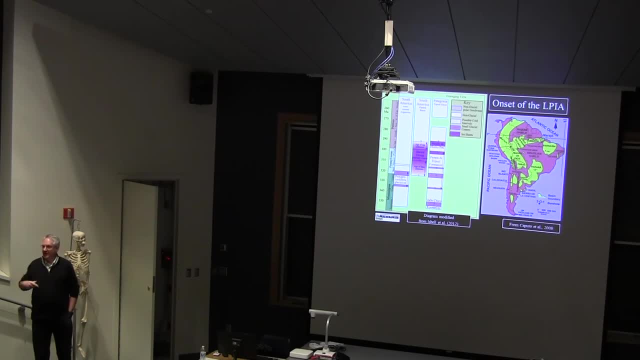 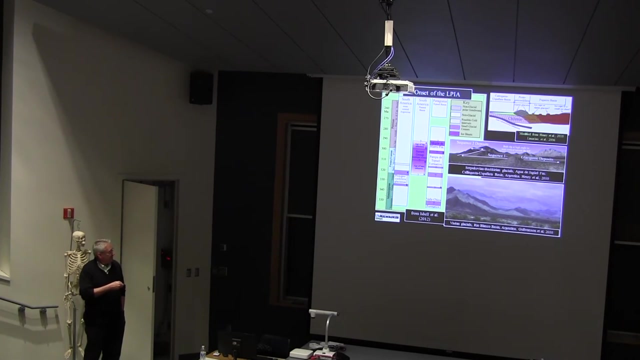 And it's really only known from South America at that time. Rocks of that age in other parts of Gondwana are not glacial, So glaciation starts in this part of South America, actually this part of South America- And then, by the time we get to the Mississippian-Pennsylvanian boundary, somewhere around 220, or 323 million years ago, 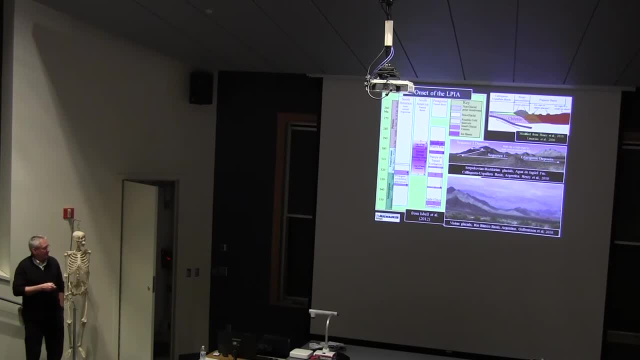 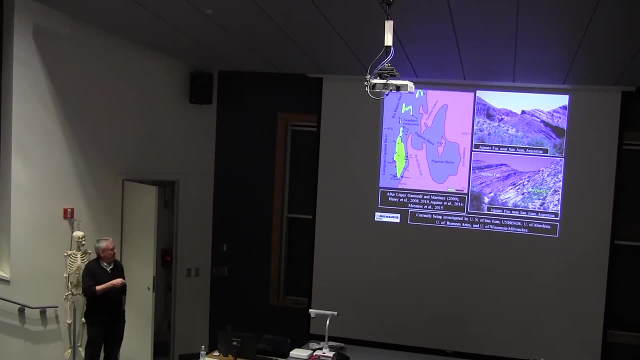 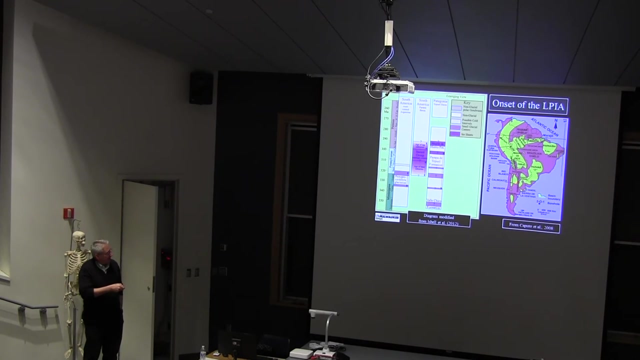 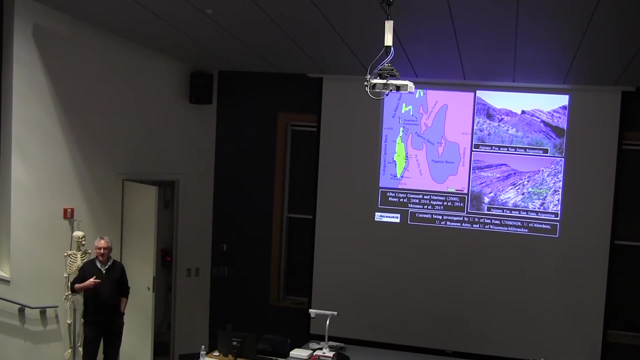 glaciation just takes off and it becomes really widespread, And it becomes glaciation primarily in the westernmost part of Argentina. So this diagram that I'll show you is this area right here in westernmost Argentina, And this is an area where there are a lot of big deep paleo valleys. 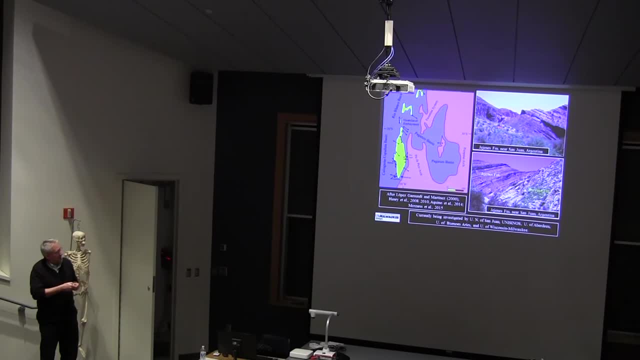 And here's the edge of a paleo valley. This one's about two kilometers across. Here is the San Juan limestone. Over here these are glacial and post-glacial rocks kind of lapping onto that basin wall. You walk across this pile and get to the other side, and this is the San Juan limestone. 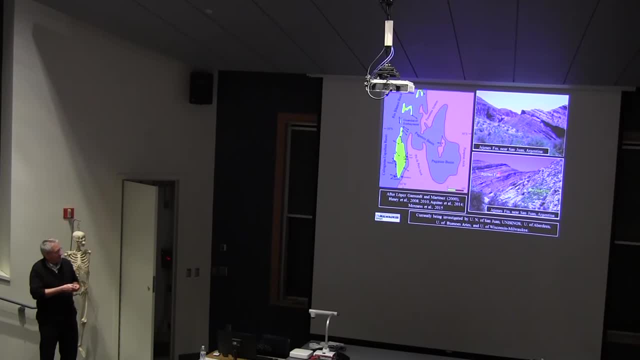 And here is the glacial at the bottom and then post-glacial, And they're sitting there and they're filling up these valleys, these very deep valleys that are up to 1,000 meters deep. So they're sitting in probably paleo fjords, the deposits. 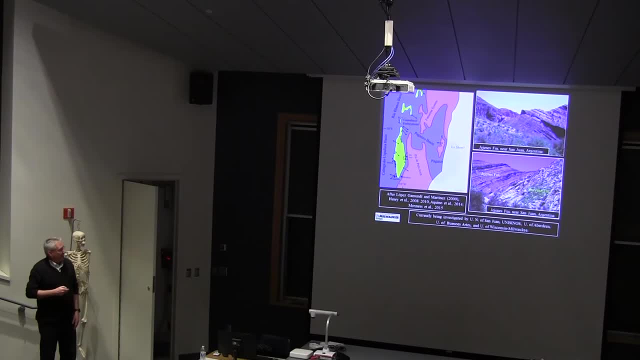 And they all occur over in this region. Kate is really interested in this area over here And there's been a lot of arm-waving saying that, well, these are outlet glaciers. The problem with outlet glaciers is some of them flow in the wrong direction. 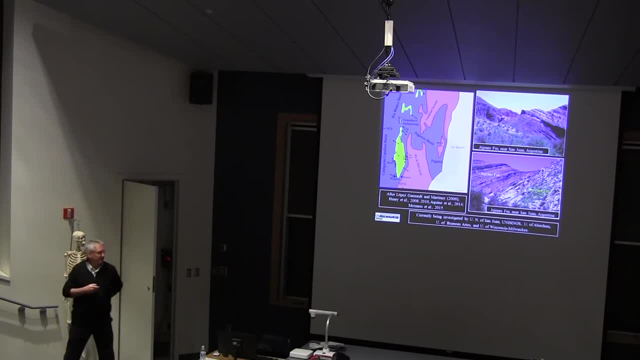 They seem to be radial away from a highland, something called the Proto-Precordiera, And there's this little area over here that people have used to say the evidence from a paleo valley over here. they've used to indicate that there is this huge ice sheet sitting over here. 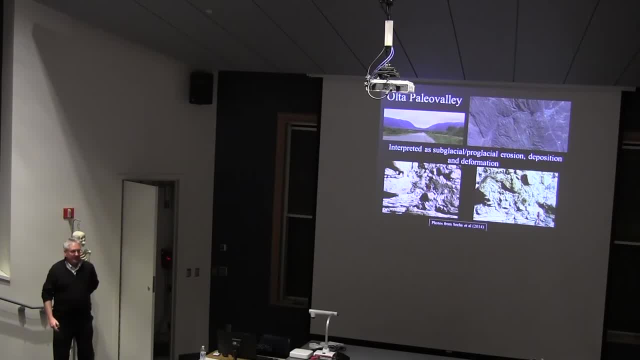 draining stuff off to the west And when Kate and Levi Moxnes last year went to this area and they started looking at it. here's the old, here's the modern valley. This is a valley called Alta Melanzan. This is actually the Melanzan part of that paleo valley. 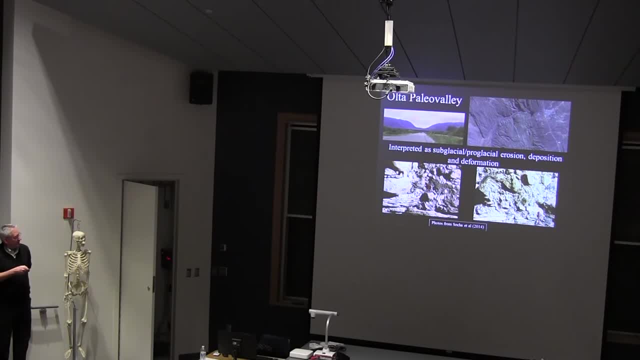 And the person that worked on this said: oh, it's a beautiful U-shaped valley, It's glacial And the only problem is that the granite walls disappear here and here And this is filled. So you can't really say that that's the shape of the valley. 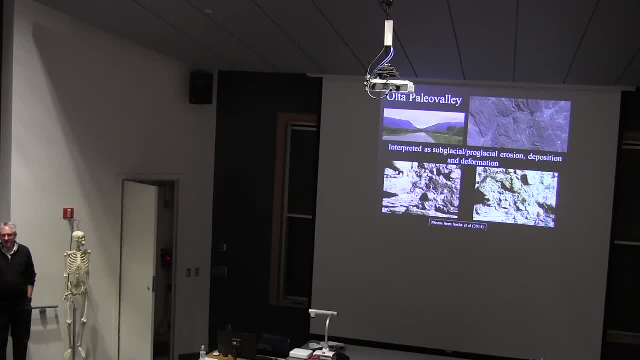 because the valley could just as easily be V-shaped And so you really need to look at the deposits within the valley and try to get a handle on how it was cut. So here's that valley, And we spent a lot of time looking at the rocks throughout this valley. 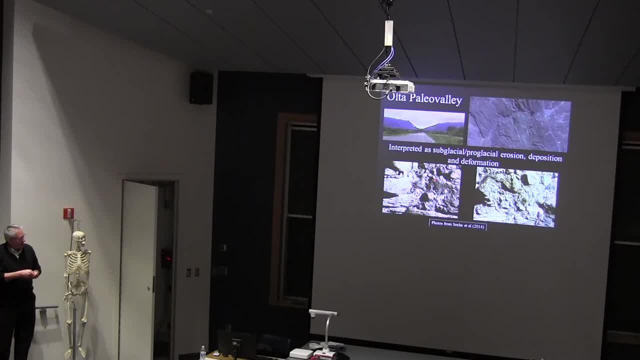 And the person that looked at these. they saw these types of deformed material adjacent to big boulders. There was a boulder sitting here And they say that, well, that's glacial shub, Okay. So when you go out and you look at the valley, 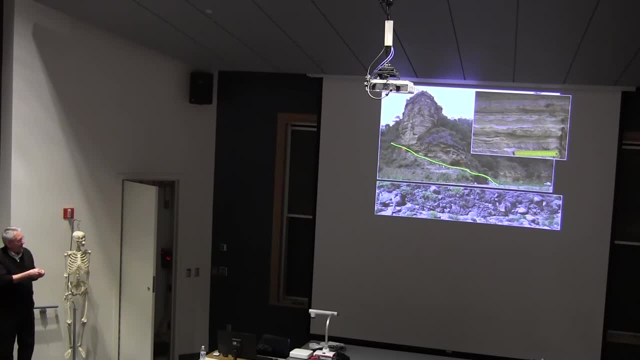 here is the valley wall And the stuff that's sitting on top of the granites and the schist in here. the fill of that is quartz, aranite, And there are beautiful wave ripples in it And there are things that tell you that there were these currents coming out. 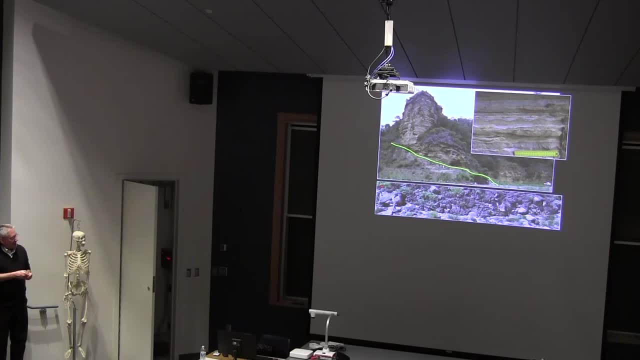 and reworking them. And there are big alluvial fans that come out into this valley And here you can kind of see it interfering with some of that sand which is a lake deposit. So these are alluvial fans prograding out into a lake. 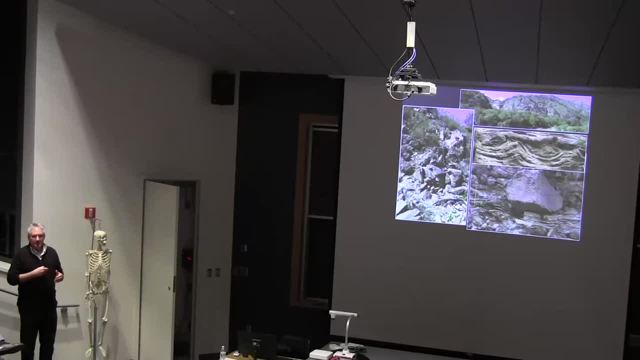 And here is another fan. The beauty about paleo valleys is oftentimes paleo valleys are the position of modern valleys, And so here's a little side valley coming into that valley And here are the conglomerates, the alluvial fans that prograded out into that valley. 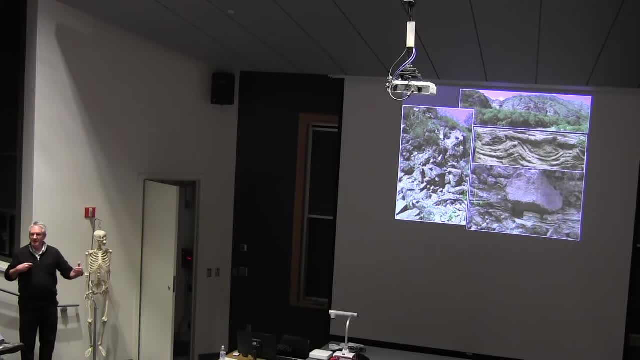 And the valley is only in some places, only 100 meters wide or so, And the valley walls are almost vertical. Here are large angular boulders. They are deforming sand from that lake. There are trace fossils in these sands that are squished. 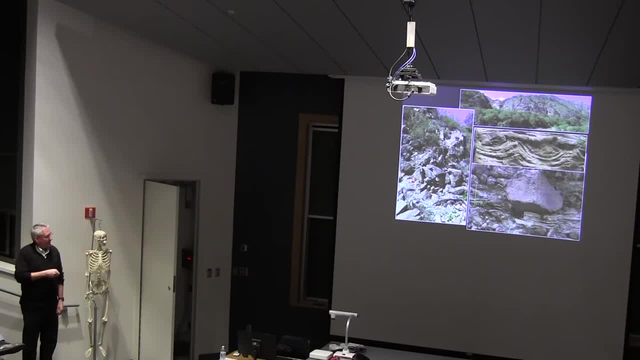 And it's not a glacial evidence. This is a landfall. It's a collapsed feature. It's a collapsed feature from the valley walls And those little push structures. here's that one that was thought to be a glacial push. 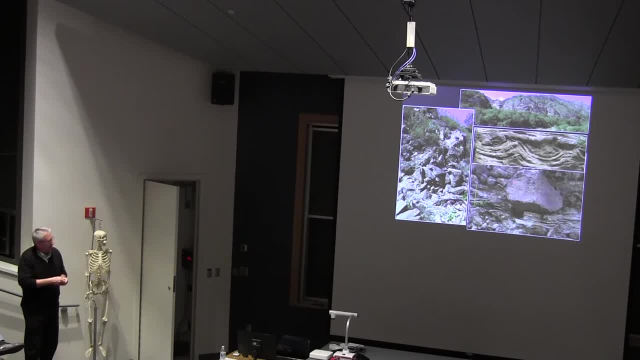 When you find and look at that there's one here and there's one here. this boulder is dropped in, So it could be a drop stone. The only thing is 20 meters in this direction is a vertical wall. This is glacial material. 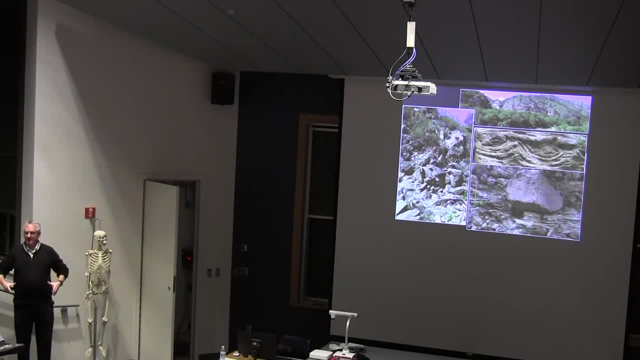 These are things that are falling off the side of the wall into the lake deposit, The bottom. Other things that were thought to be glacial shoved structures turn out. they are seismites. They're the result of failure and liquefaction and escape of water due to earthquakes. 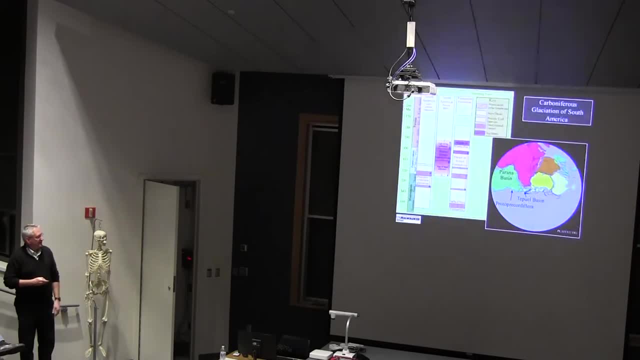 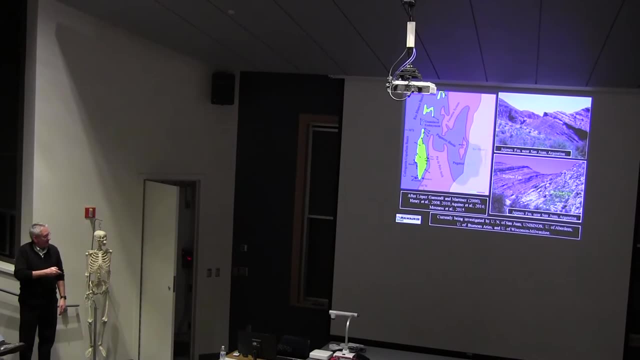 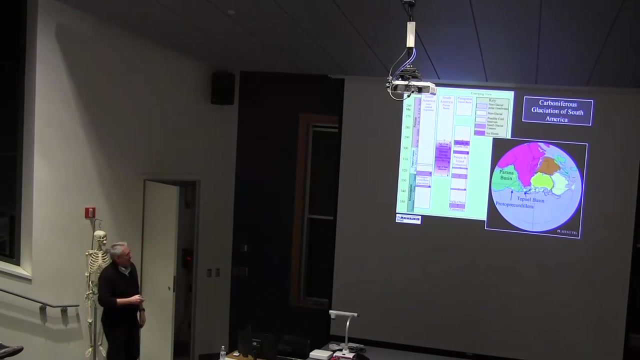 They're not due to glacial activity. So that whole concept of having an ice sheet sitting over here really falls apart when you look at the evidence. Thank you, So that time frame was the same time that the glacial valleys in western Argentina were occurring? 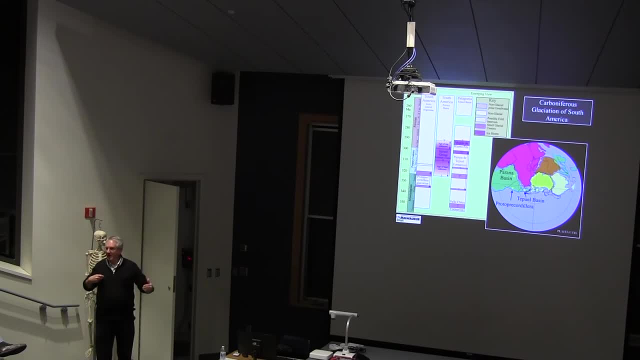 The glaciers disappeared in western Argentina and they're gone In this region. they haven't come back. When you go into the Andes a little ways away, yes, there's Cenozoic glaciation, but glaciers disappeared at the Mississippian-Pennsylvania boundary. 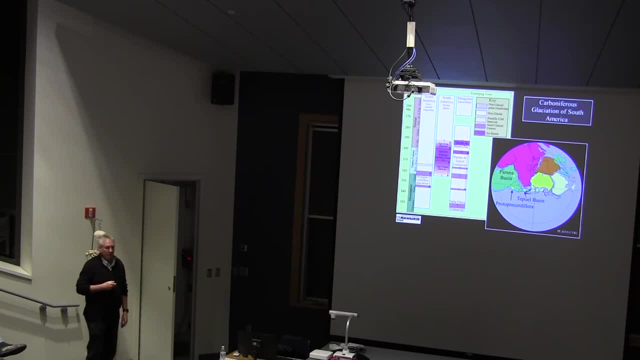 and they're gone for the next 320 million years. But when you look and you go from that area and you go actually a little bit farther away from the pole into the Paraná Basin in Brazil, Brazil's got glaciers and they're just cooking away. 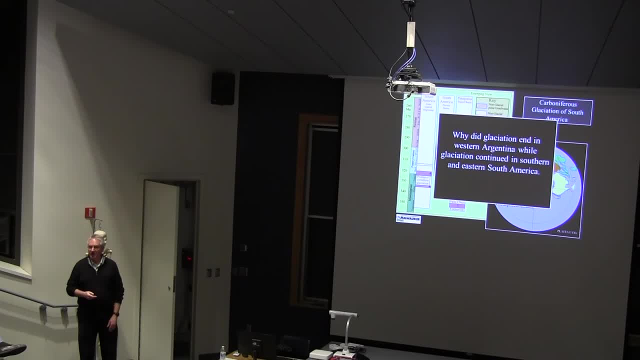 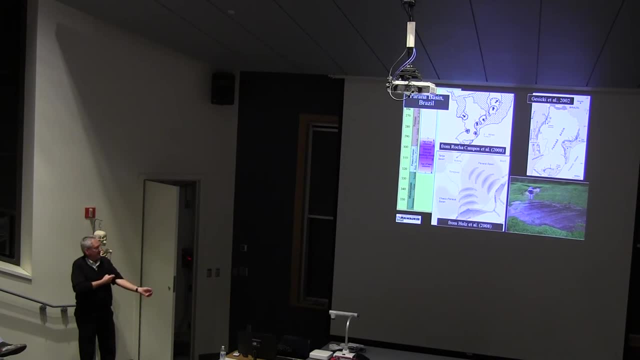 So that's a big question: Why was glaciation occurring elsewhere, at a position just a little closer to the equator than they were in western Argentina? And the big question there is: how big were the glaciers? There's a lot of hypotheses. 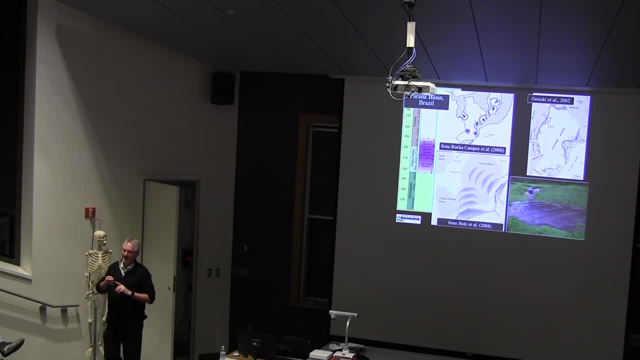 The biggest hypothesis- well, the two biggest hypotheses- is that that Antarctic-centered ice sheet extended all the way across Brazil. The other is that there was glaciers extending out of Africa, which is located here, and extending out into Brazil and making it all the way across. 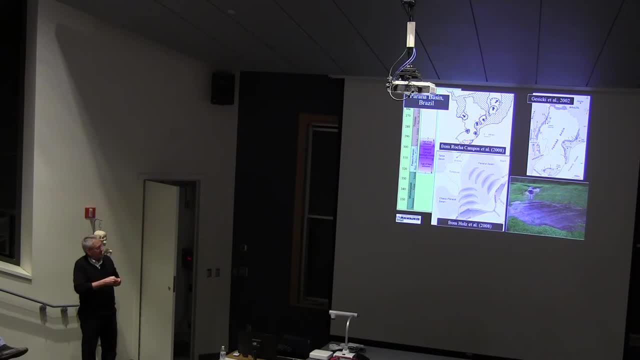 into Paraguay and Bolivia. The other hypothesis is you had little ice sheets, little glaciers setting along the margin of the space and feeding ice into it, And that's really important because this is going to require a really large ice sheet and the melting of that ice. 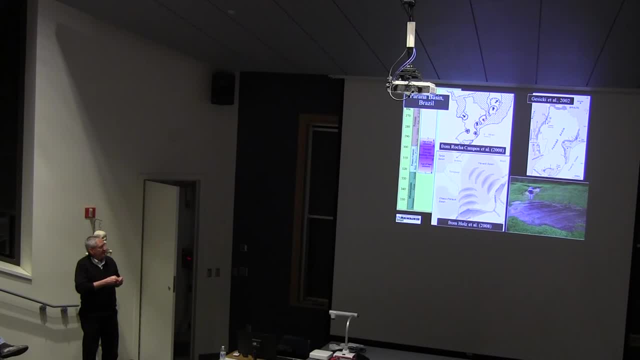 produces dramatic changes in sea level. These glaciers, they're big, but they're piddly when it comes to changes in sea level. You're talking about a half a meter or centimeters instead of tens of meters, depending on the size of the ice sheet. 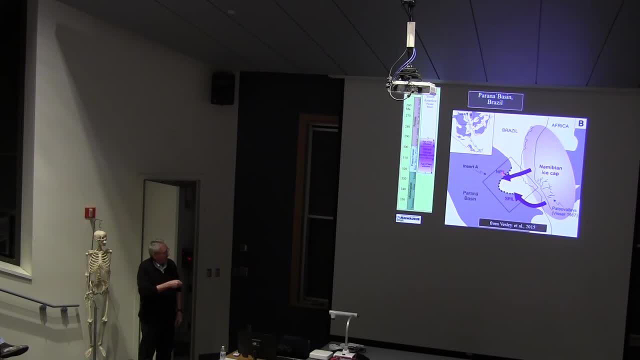 So another view of what one of those ice sheets coming into southern Brazil may have looked like. So this is in that incest. The other thing is it's thought that those glaciers advanced back and forth across southern Brazil into somewhere around about 292 million years ago. 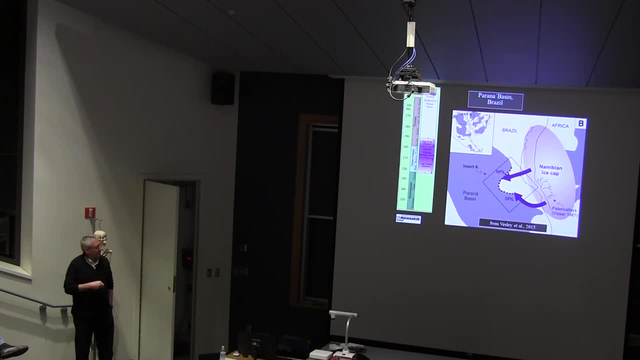 And within the last couple of months we've dated some of the ashes- Our colleagues at NASA, at the University of California Davis- And what we find is that those glaciers were older than the Permian. They are older than 300 million years. 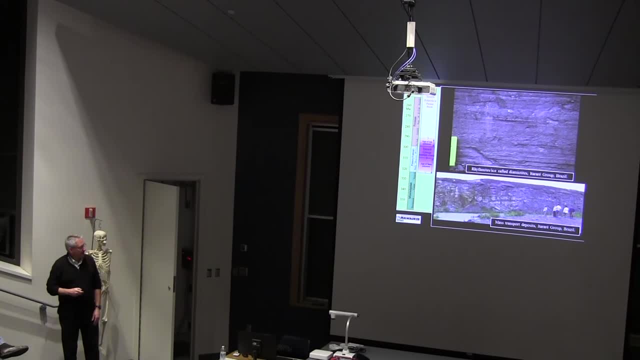 So the record is dramatically changing as we look at it. Here's some more of that succession. There are arrhythmites, There are dropstones throughout this, But this is getting out into the basin. This is often thought to be subglacial in here. 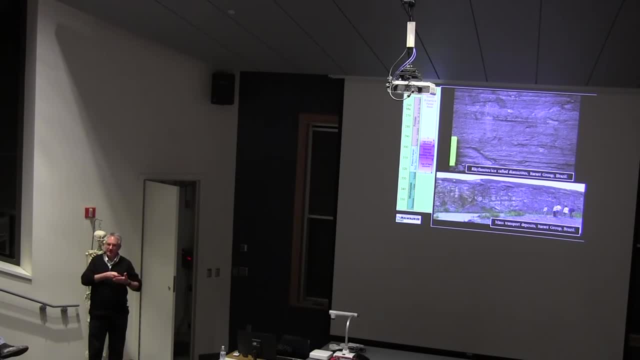 But these are large slide blocks that are sliding down what's equivalent to a continental slope at the edge of a continental shell, and not stuff associated with glaciation. So we're really struggling with the size of these glaciers And they don't appear to be as big as they were. 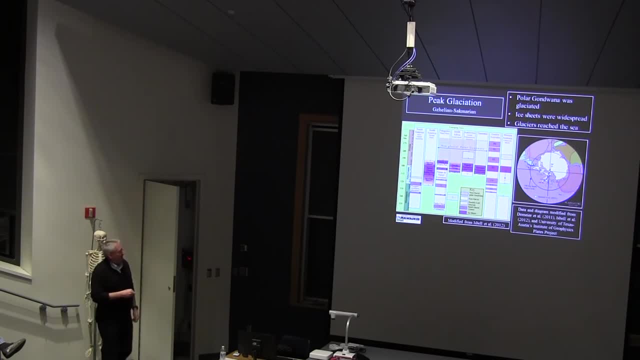 And the timing is certainly not as long as it used to be. So now let's jump into the end of the Pennsylvania and into the Permian, And at the Permian there's evidence that there was glaciation everywhere in Gondwana. 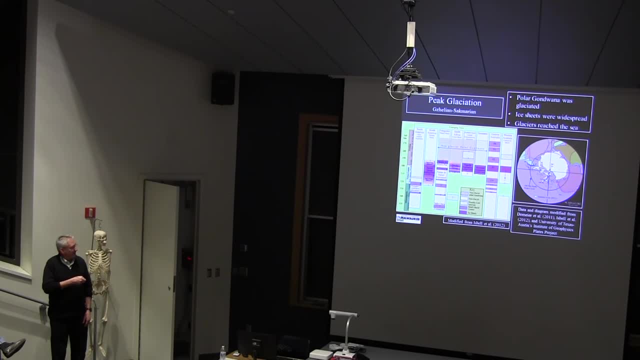 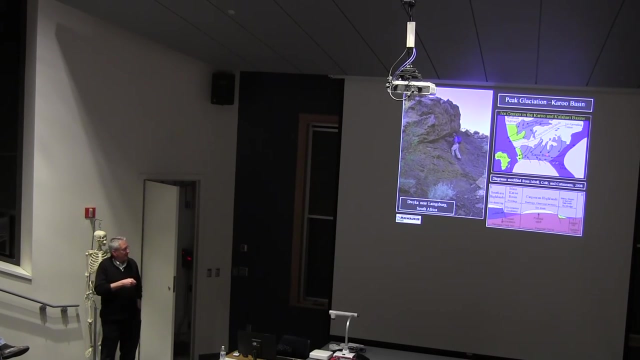 that it extended from southern Africa- maybe southern Brazil, excuse me- southern Argentina- and Patagonia across southern Africa, Antarctica, India and Australia, And it's thought that this was the most widespread point of that glaciation. And here's some stuff in southern Africa. 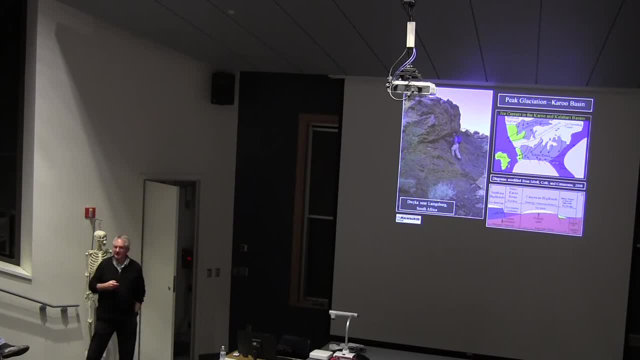 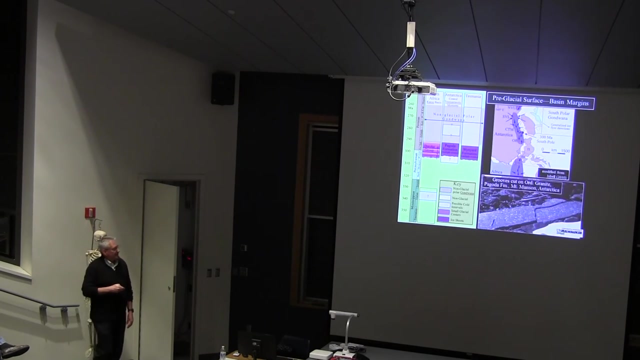 And the flow lines indicate that there are more than one glacial center. So it's not a big ice sheet extending out of Africa, But there are smaller ice sheets in Africa that are pouring ice into what's called the Karoo Basin. Then we jump to Antarctica, my favorite place. 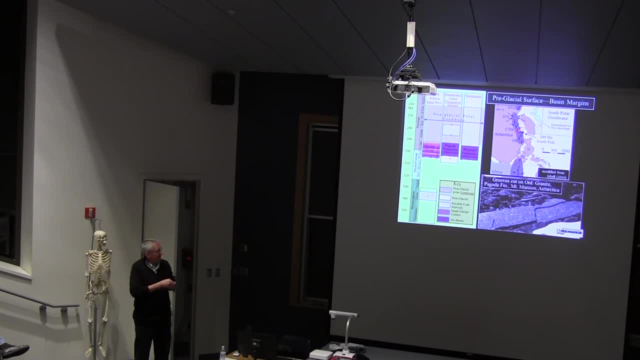 And this is the area in here, the Transantarctic Basin that Bill and I work on. Bill works primarily in the Triassic and Jurassic. I work primarily in the Permian in here, And this is the shape of that basin. at the time there were glaciers. 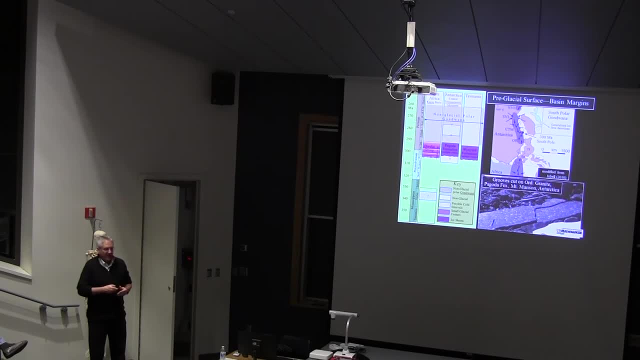 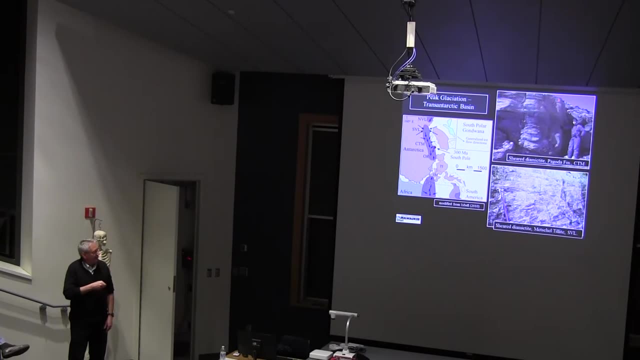 There are basement rocks that are striated, And glaciers do striate basement rocks. There are things that are highly sheared, That look like they were overridden by ice, And here's another one. And when we start plotting out flow lines, what we find is that the glaciers 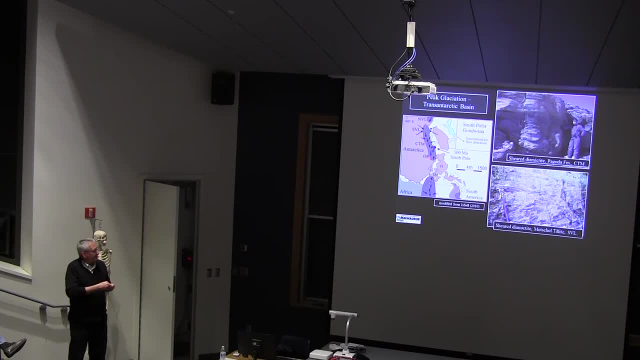 evidence for glaciers occur along the margins of this basin, But by and large they only occasionally extend into the basin and then flow down it. But what that suggests is that there was ice sitting over here, and ice sitting over here Instead of one big ice sheet that was located over the South Pole. 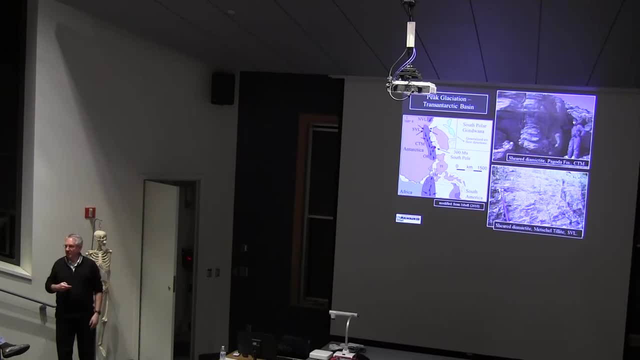 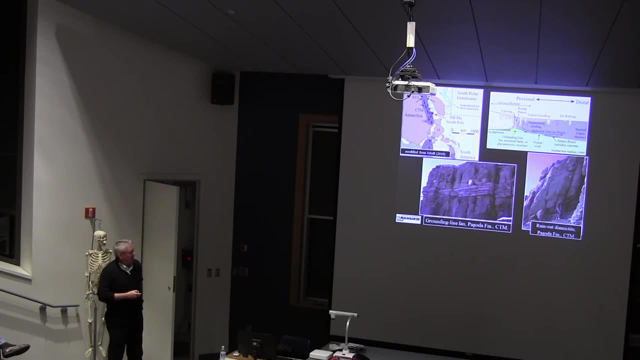 and extending out over Gondwana. Antarctica had multiple ice sheets, As did South Africa, As did South America, And then there's evidence within the basin that you get these wedge-shaped sandstones that show evidence for water coming out into this area. 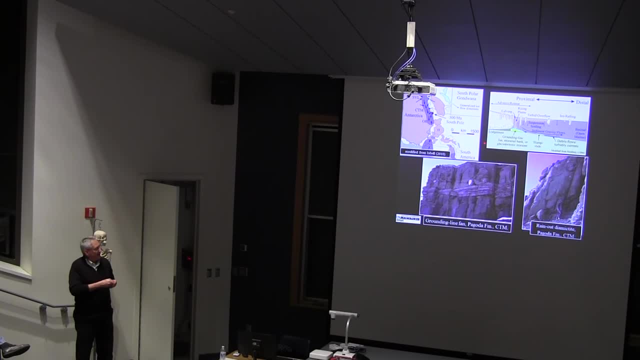 and then beginning to float, Suggesting that it may be some type of meltwater plume, And then you've got these big stones that appear to be dropped in Sea- ice- icebergs, But this is out here in the basin. 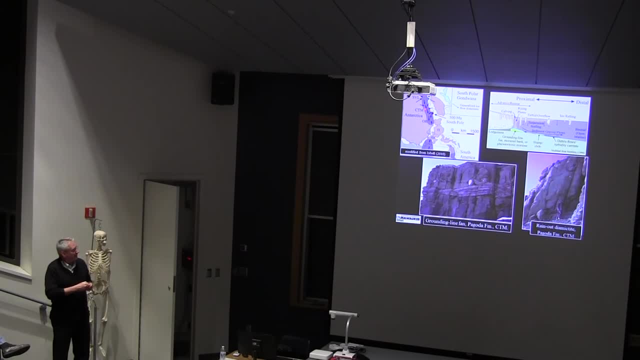 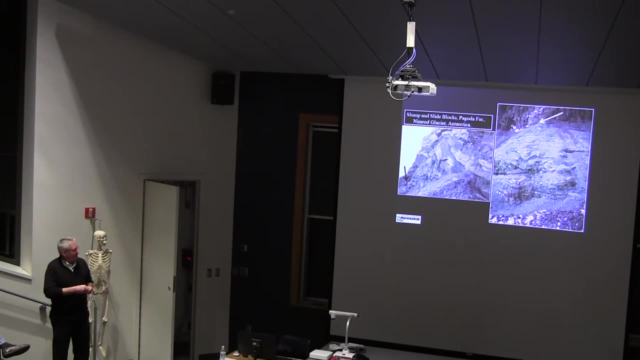 and there's not a good set of evidence suggesting that the glaciers were overriding it, but they were sitting nearby. And then there is again lots of evidence. These are: You can see a big block that's slid. This is sliding down the basin slope. 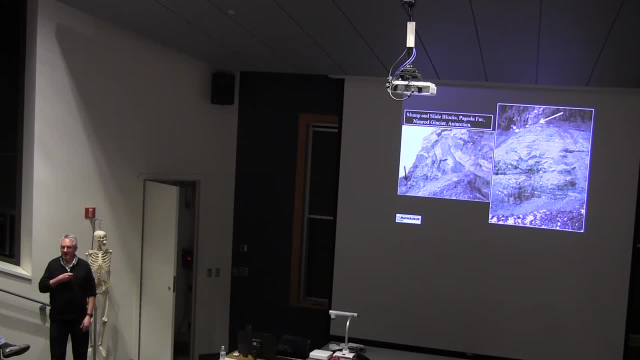 that's essentially equivalent to a continental slope, So there's a lot more than just glacial activity going on. Here's a person to scale- This person's only about this tall, though- And then there's another person up here to scale. 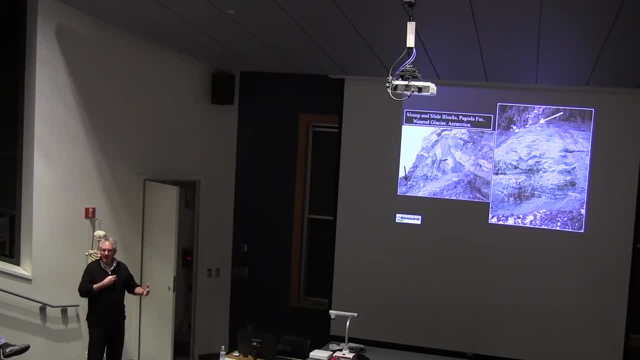 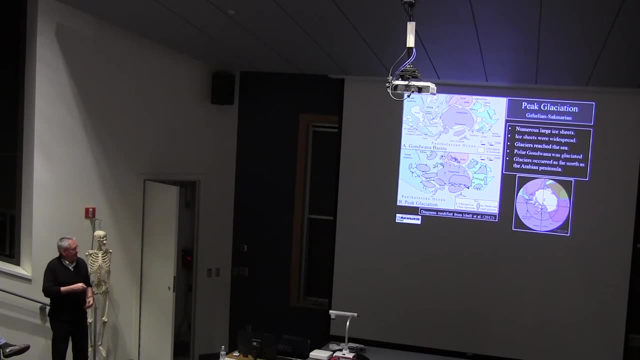 And here's some folded strata, the result of sliding and slumping, But not necessarily glacial activity. So when we look at peak glaciation, this is what we think is happening: that there are lots of glaciers and that they're growing and shrinking. 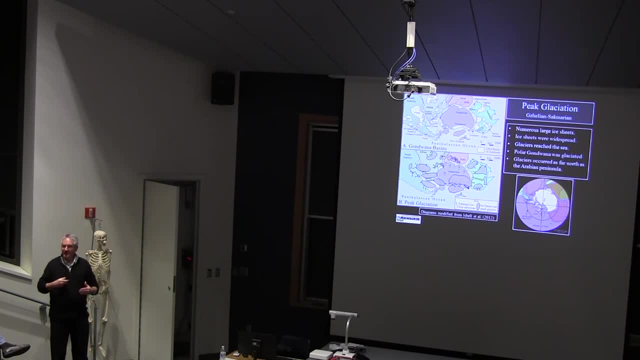 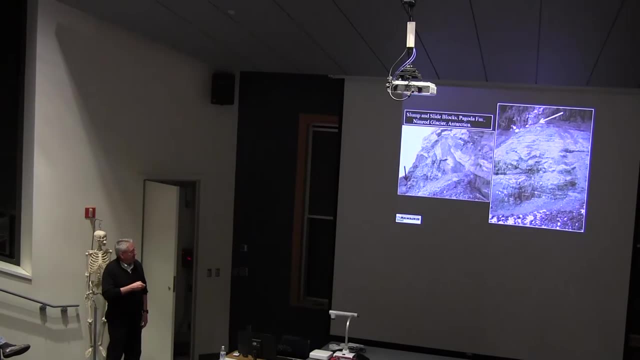 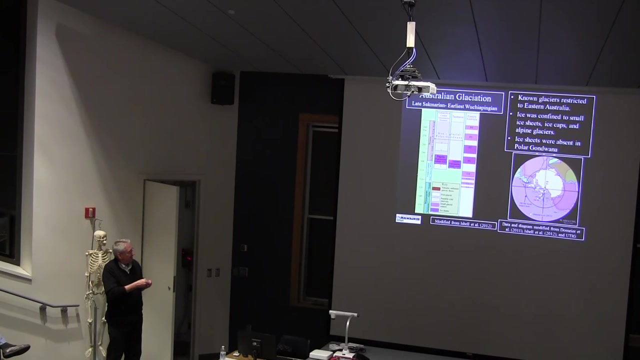 and responding to global climate, but not a single large ice sheet. Then when we go past peak glaciation- which peak glaciation is right in this area? Here is the Antarctic deposit, Tasmania. When we go past that, and there are also stuff in Australia. 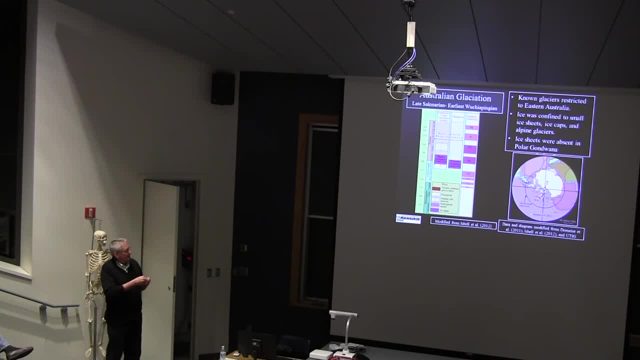 in that peak period. when we go past that and we start looking into the later Permian, there are glacial deposits, or things that have been interpreted to be glacial deposits, sitting over in here. They're in the mid-latitudes, But at that time 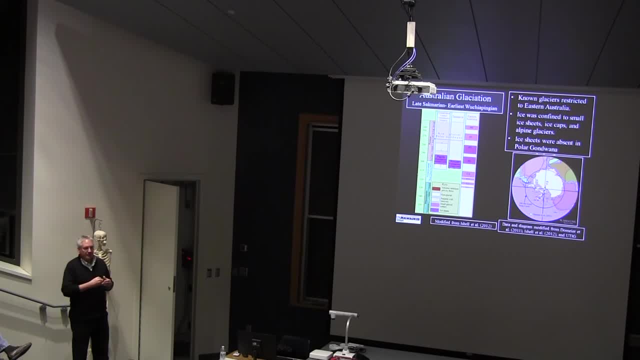 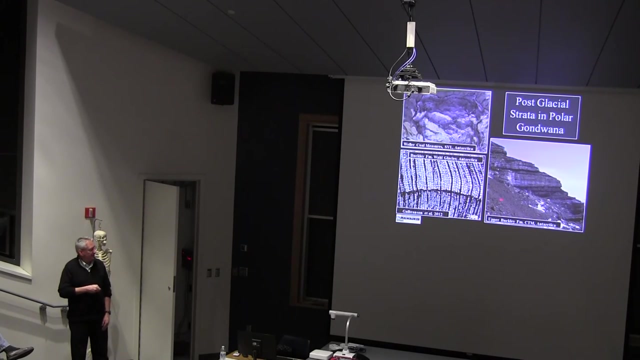 here is the polar circle. The polar circle appears to be ice-free And at that time, when you look at the deposits that were occurring in Antarctica, that was sitting within a degree or two of the South Pole. this is what you see. You see extensive deposits of sand and coal. 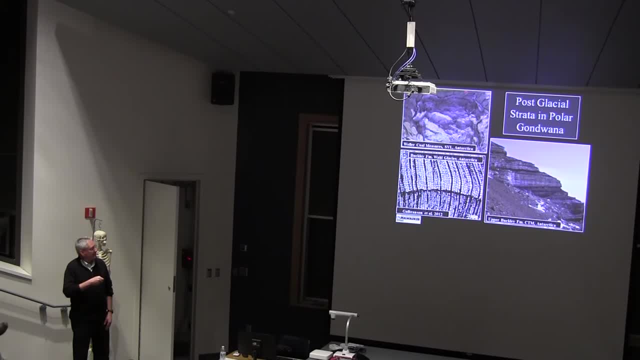 The plants show good evidence for growth rings. So here's a big stump and you can see the rings in it. When you look at the rings which are preserved, there's no evidence for frost damage during the growing season And geochemically. 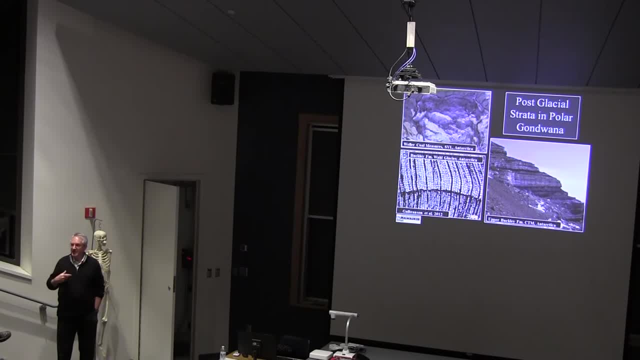 the type of growth that they appear to be experiencing is more typical of what you would see in the Pacific Northwest rather than in a polar setting, even though they're sitting at the South Pole. So there's this big problem in: why are there glaciers at mid-latitudes? 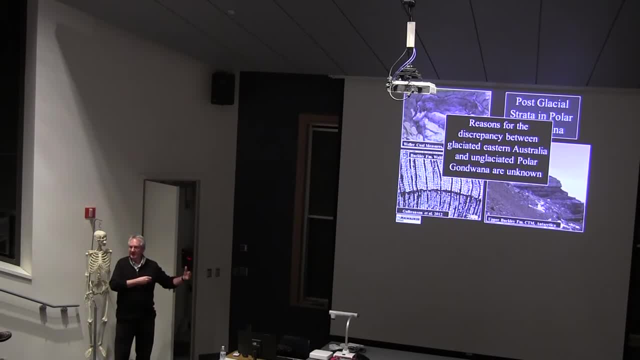 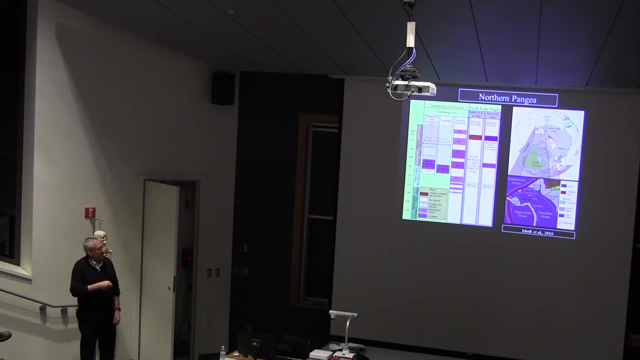 They're small glaciers, and why wasn't the pole glaciated at that time? Okay, let's jump to the Northern Hemisphere and look at the possible bipolar glaciation During this timeframe, during the Pennsylvanian and Permian, Pangaea was drifting northward. 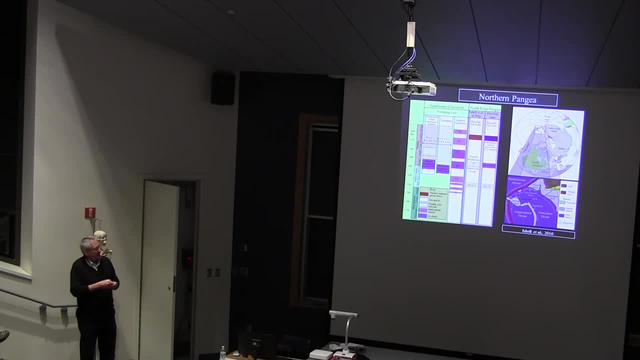 and it was drifting into the North Polar Circle and Siberia, ultimately drifted across the North Pole by the end of the Permian And this is blowing up this area. There are areas where these yellow triangles are showing you where dimictites occur. These are all in deep water basins. 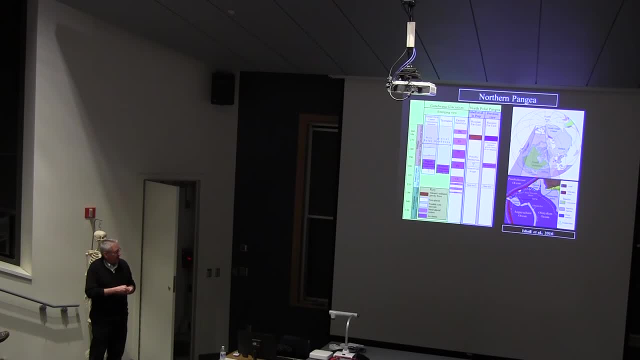 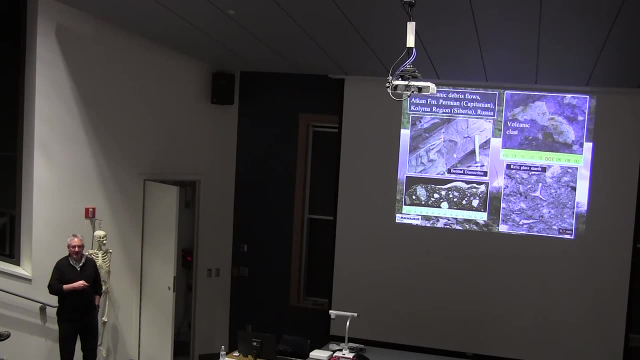 and they're sitting adjacent to a volcanic arc. And when you look at the composition, these are the dimictites. They're all bedded. They have the characteristics not of glacial deposits but of debris flows. You cut into them and here they are. 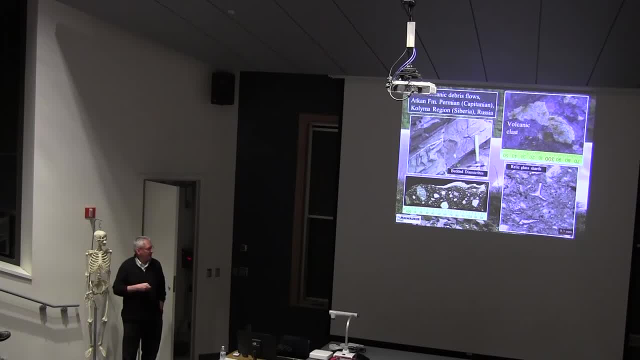 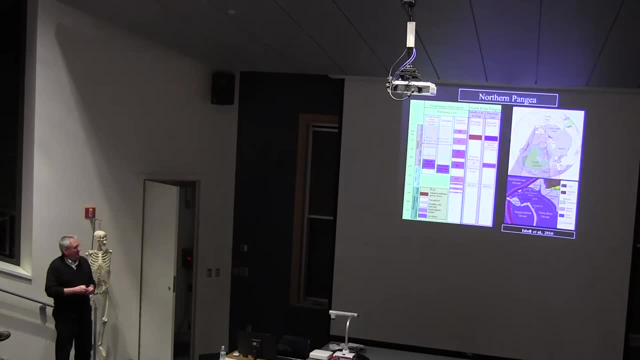 It's chock full of volcanic material And the matrix is chock full of material that has glass shards, So we're interpreting these as being volcanic debris flows, And so we're no longer thinking that there are glacial deposits at that time, but all the material is coming from a volcanic arc. 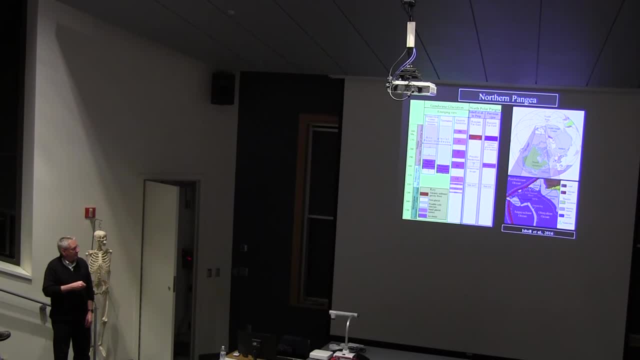 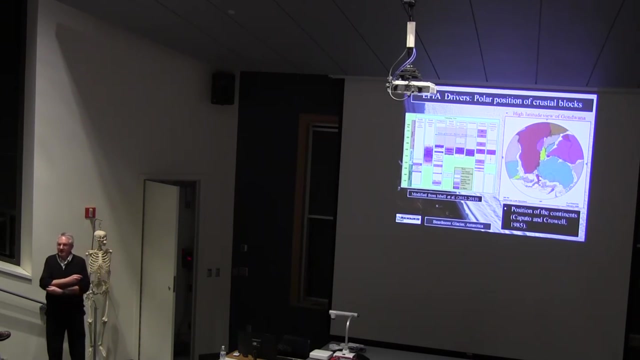 into these deep water basins, So we would change what we thought was going on in the Northern Hemisphere And at this point there is no evidence that there was bipolar glaciation going on. So let's look at some of the drivers, Because they're pertinent to us. 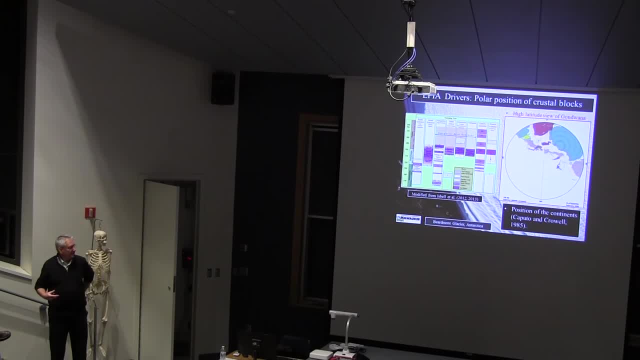 First off, one of the early ideas was that well, Gondwana and Pangea moves around through time. So here's the shift of Gondwana across the South Pole, The South Pole being located here And going from initially the Devonian. through the Pennsylvanian into the Permian, and then even a little younger, And so it was thought that Gondwana just drifted over the pole and then off the pole, And that was why glaciation started and that's why glaciation ended. 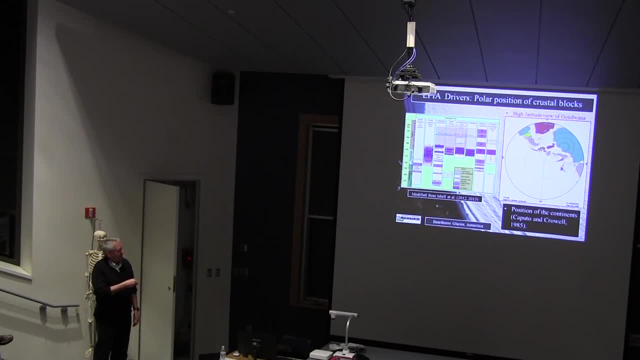 But in a general way, that's true. It starts over here in South America and then it progresses, And then it starts in Australia, and then it progresses across all of Gondwana and then it disappears in Australia over here In a real general way, yes, 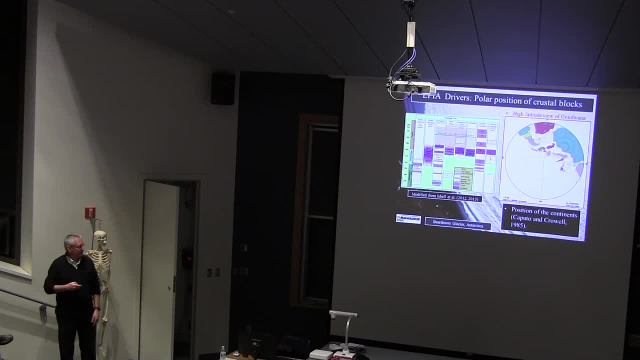 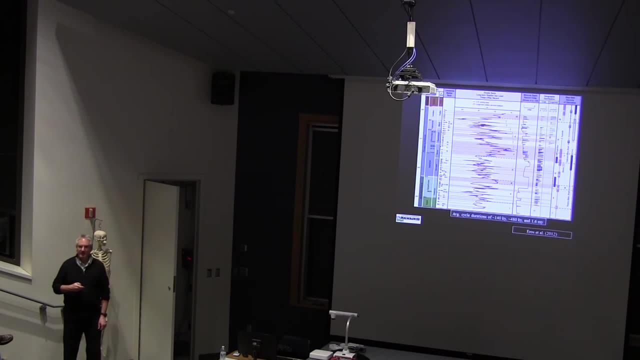 we need to have the continents in a polar position. But there's a lot more to the story. These little fluctuations in here are looking at cyclothems and the fluctuation. These are showing advance and retreats of sea level onto a continent. 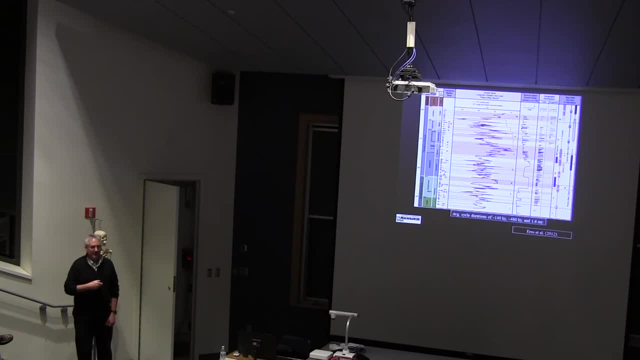 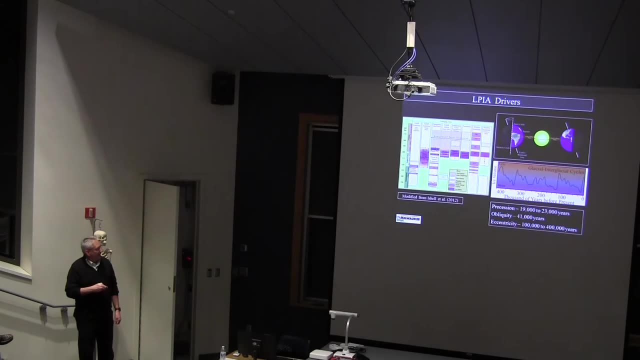 This one happens to be in Ukraine. This record is not accessible at the moment because of the problems in the Donetsk region of Ukraine, But they look very similar and are, on a time scale, very similar to orbital fluctuations. Remember, our pole is tilted away from the sun. 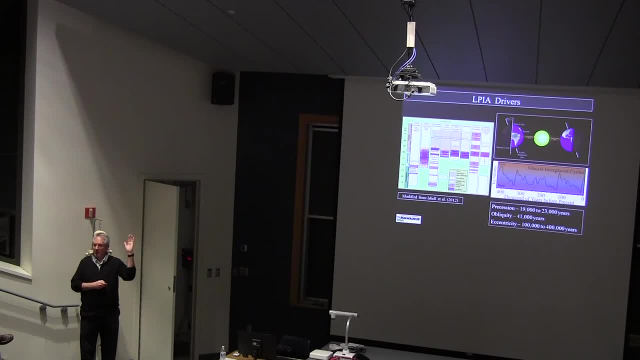 so that gives us seasons, And sometimes the pole, over an interval of time, will move back and forth a few degrees. There's a wobble to the pole And the Earth's orbit. sometimes it's more circular, sometimes it's more like a football. 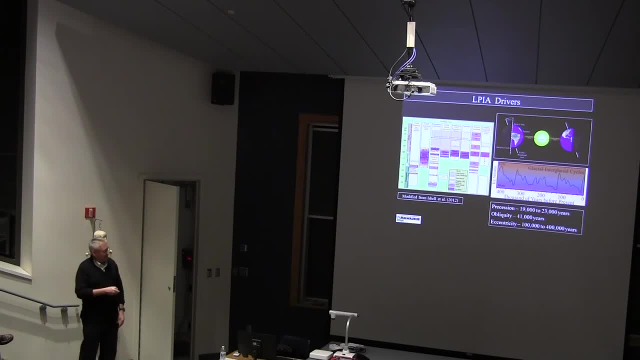 And all of those vary over intervals of time. The precession is 19,000 to 23,000 years, The obliquity 41,000.. The eccentricity, the change of the orbit, is on the order of 100,000 to 400,000 years. 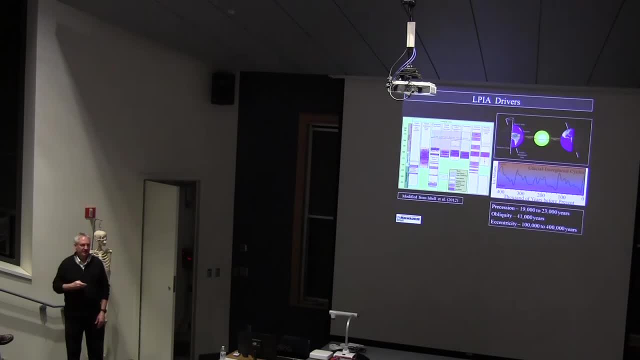 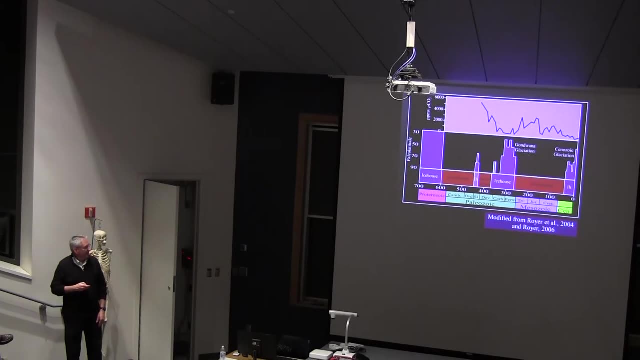 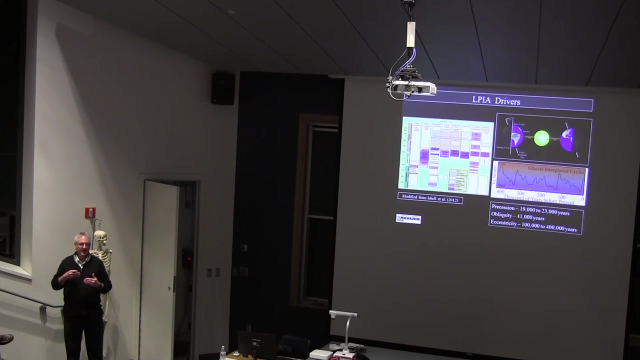 And it looks like they fit pretty nicely with this record, suggesting that, yes, there is a component of these orbital parameters driving these ice sheets, But that's within a glacial period. They're not driving the beginning of glaciation and the end of glaciation. It's fluctuations like in the Pleistocene that we see in North America and in Antarctica today: Fluctuations in the growth and decay of ice sheets because of changes in insolation. This is the long-term CO2 through the Paleozoic, Mesozoic and Cenozoic. 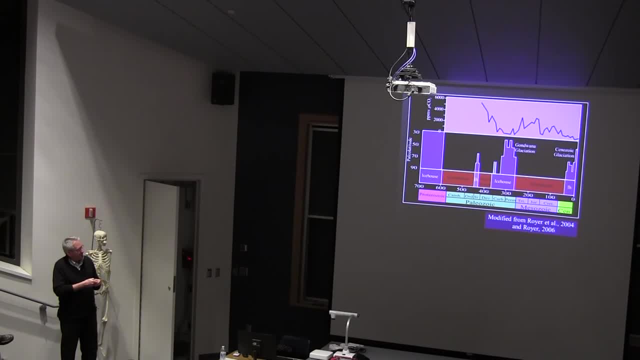 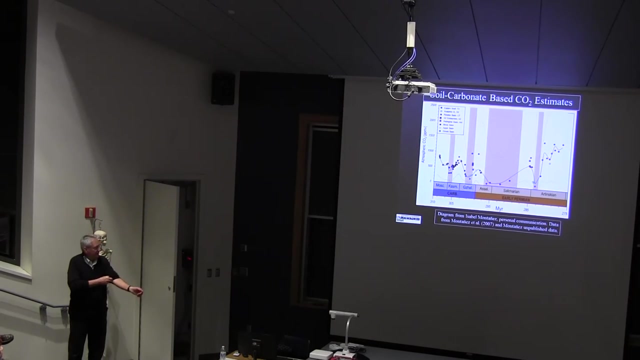 And the Late Paleozoic Ice Age is a time of low CO2,, as is the Cenozoic Ice Age, And then CO2 rises A little more refined work. So this is the work of Isabel Montanez. She and her students are helping us. 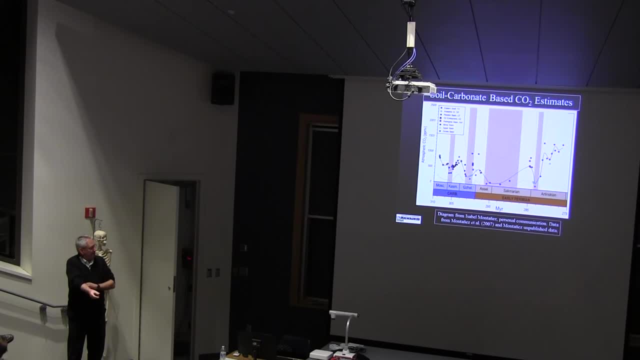 with the work in Brazil And she looks at soil, chemistries, Paleozoals, And she tries to extract CO2 record And what she finds these are the time frames when we've got glaciers, that there are dips in the record. 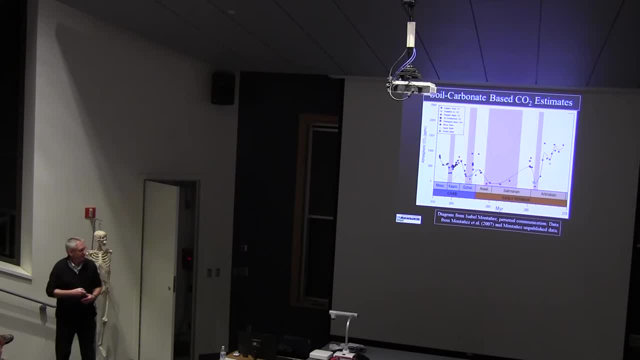 So there are times of apparent low CO2. And then, when we go into a non-glacial record, there seems to be a rise and so forth, And that when we have this rise, that's when we come out of these glacial periods. 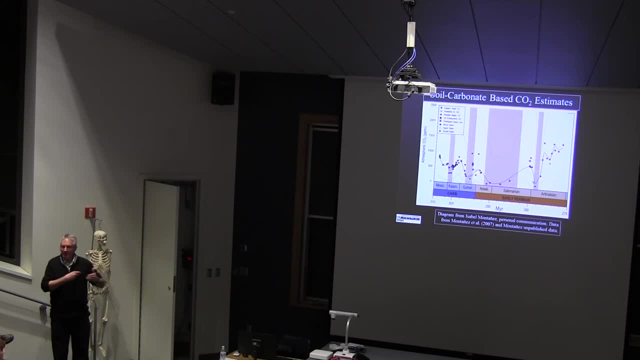 So in here there would be lots of these orbital fluctuations. But then we rise out of a glacial period during CO2 increases, fall back into a glacial period during low CO2, and then come out of it. Big problem is: what's driving this CO2.. 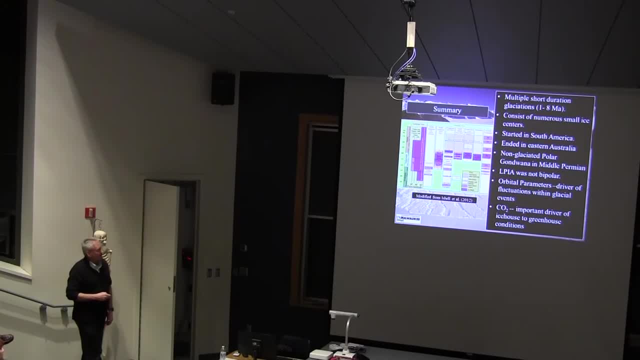 She doesn't know, and I certainly won't suggest that I know. So just to sort of summarize all of it up for the late Paleozoic, it doesn't appear to be a single large ice sheet that lasted for 100 million years. 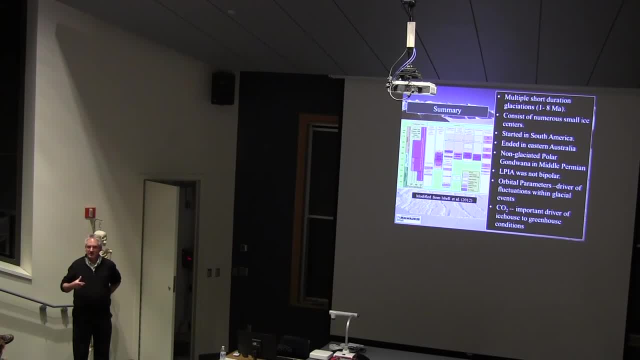 but numerous ice sheets, small ice sheets that had durations of a few million years, separated by non-glacial intervals of a few million years. They started in South America, in the Devonian and ultimately ended in Australia in the Permian. When it ended in the Permian, Antarctica was in a polar position, as was South Africa was just on the edge of that polar circle. Tasmania was just on the edge of it. Polar Gondwana was not glaciated at that point, So it's a really complex history. 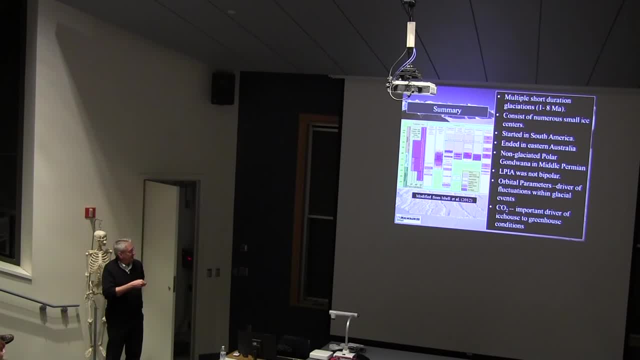 There are orbital parameters that suggest that there are fluctuations going on within that ice age and it looks like it's CO2 that actually is what causes the beginning of these major glaciations at the end and then the end of the whole late Paleozoic ice age. 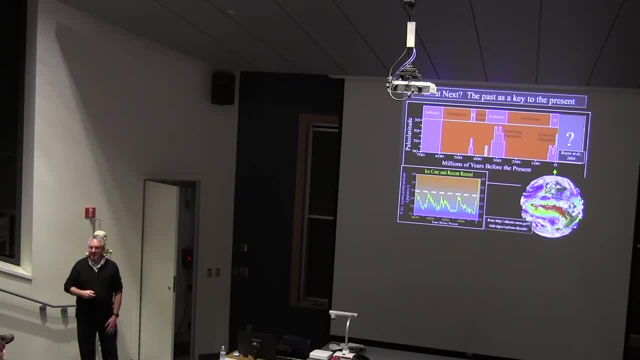 So ending here and then going into a glacial period in the Greenhouse Earth, And again our big question is: is what's happening here? So if we look at the CO2 record over the last 400,000 years here it is fluctuating. 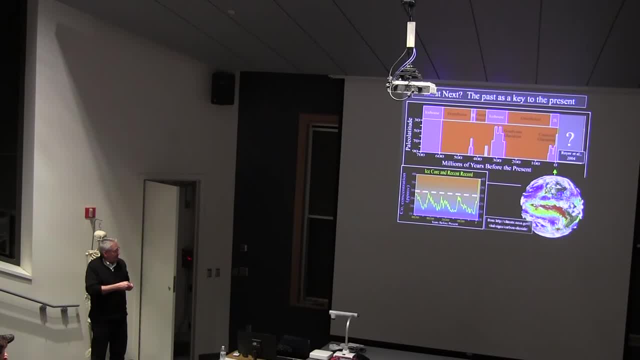 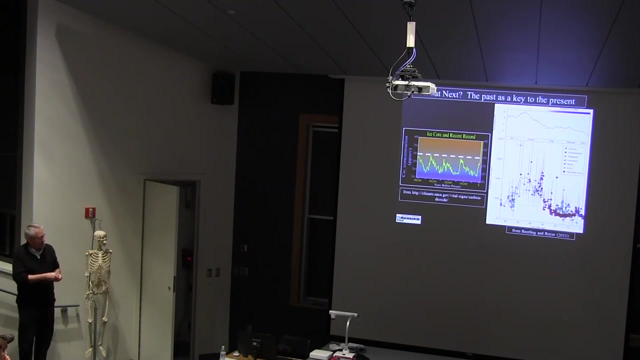 and it's fluctuating with ice volume and temperatures, and CO2 never rises above 300 parts per thousand. We haven't been above this level prior to recently since at least 18 million years ago, So it's a long-term record. 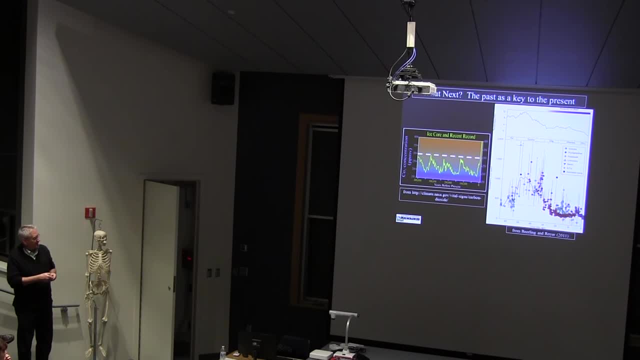 Going back into. here's the Eocene and the Oligocene and the Miocene and here's approximately 300.. There's a little blip here in the Miocene and then we've got to go back. this is about 18 million years. 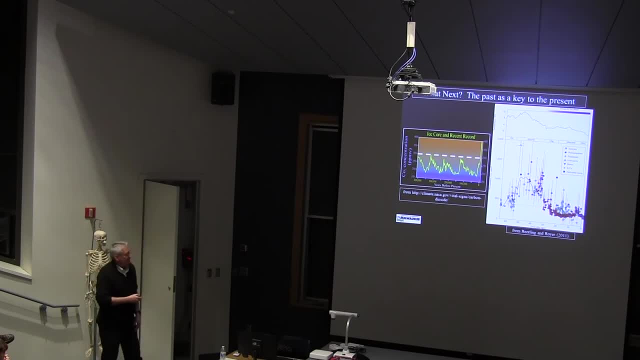 and here's the average, this line: We've got to go back into the Eocene and the Oligocene before we see CO2s that we're now seeing in here. So if the late Paleozoic Ice Age is any indication, 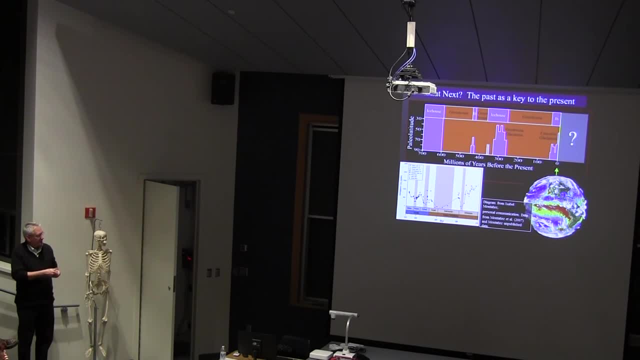 and we come out of these glacial periods when CO2 rises dramatically. we can apply that and then say: well, are we rising because we haven't been at 400 for a very, very long time and we're now at 400.. 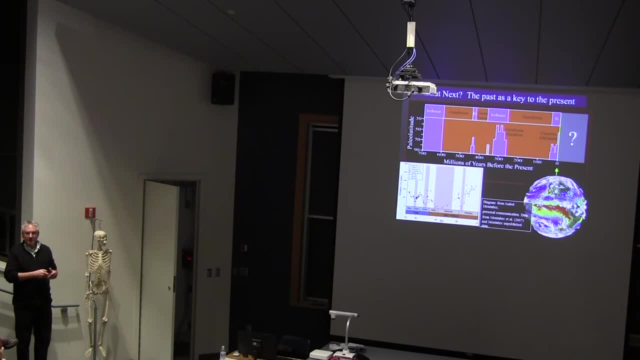 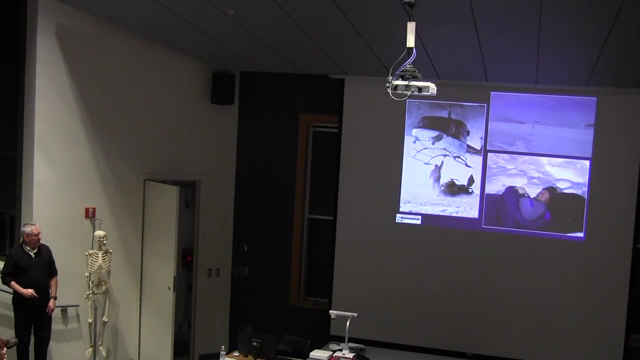 Are we actually coming out of the Cenozoic Ice Age, which we're still in, and are we transitioning into a green house era? I'll leave it there, Thank you.